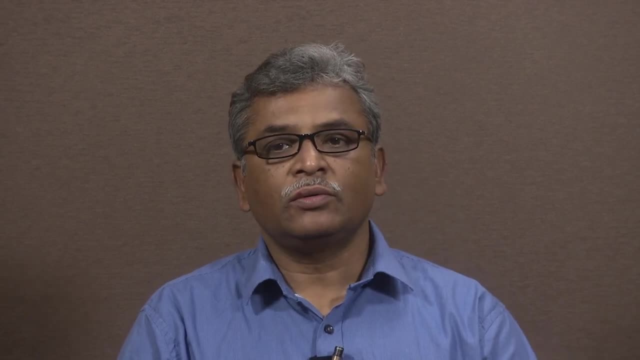 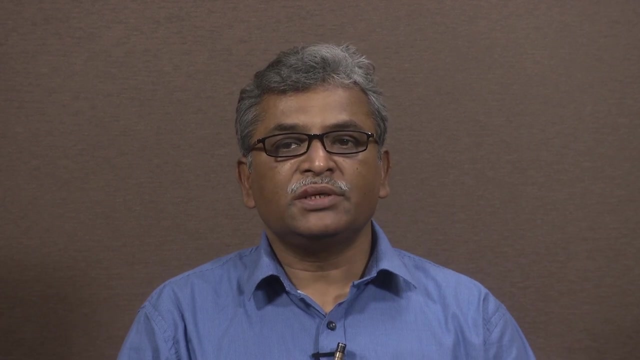 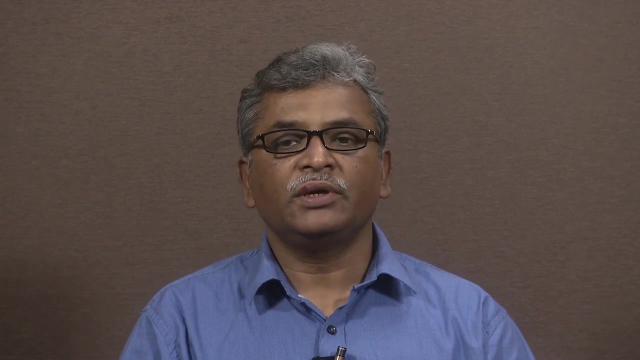 is called plate and frame filter, fish and also rotary drum filter. In that case we have discussed something about how that particulate materials can be separated. what is the basic mechanism and what is the governing equation and, based on that governing equation, how we can assess that filtration process. what are the basic components of those filtration process? 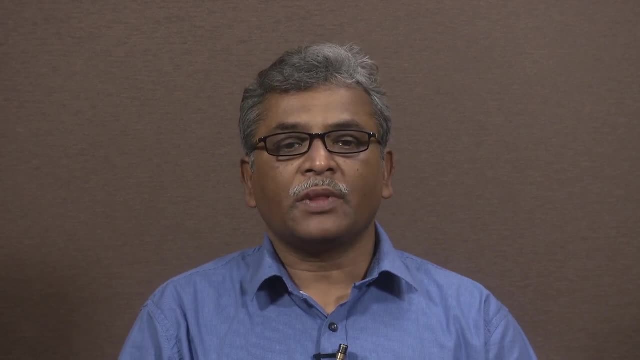 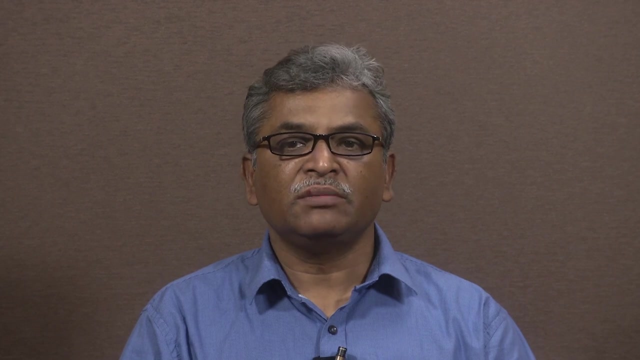 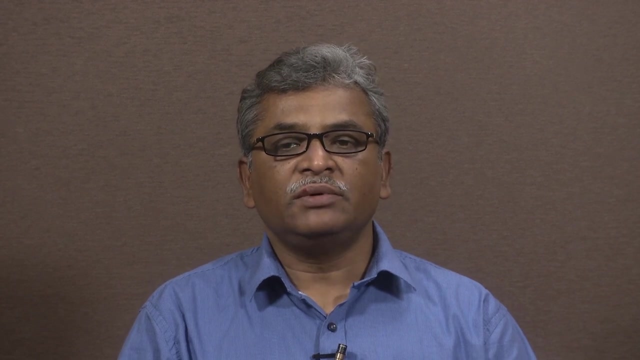 like there are some Factors, like you know: cake deposition, even specific cake resistance, even filter medium resistance, those will be actually affecting the filtration efficiency there. Also, we have discussed that rotary drum filter. there are also that some components, like you know that. 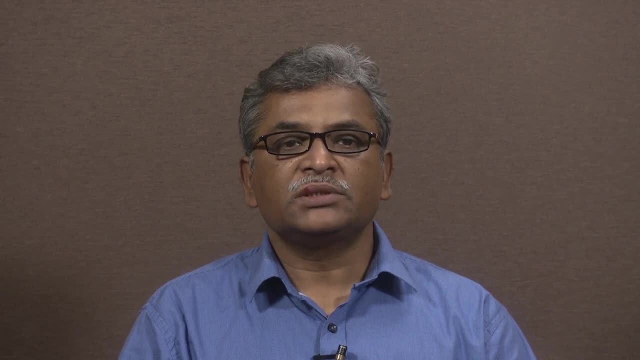 rotational speed, even filter medium resistance, cake resistance, also the submerged area of that, you know, filter, Which will affect that. you know efficiency of the filtration process. There we have calculated how to you know, there we have discussed how to estimate that filter medium resistance. 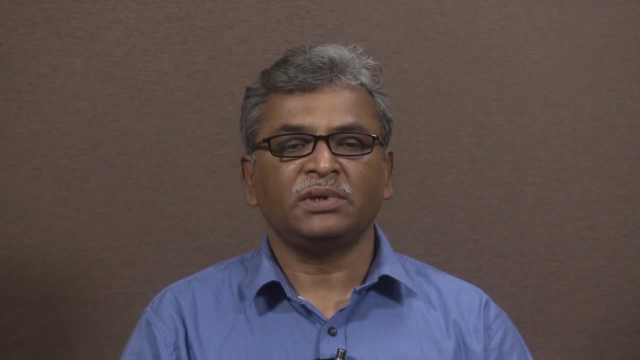 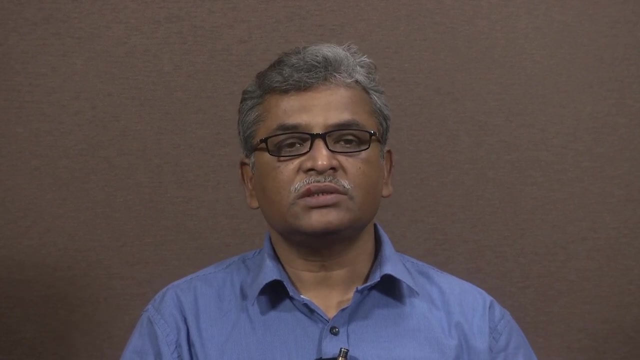 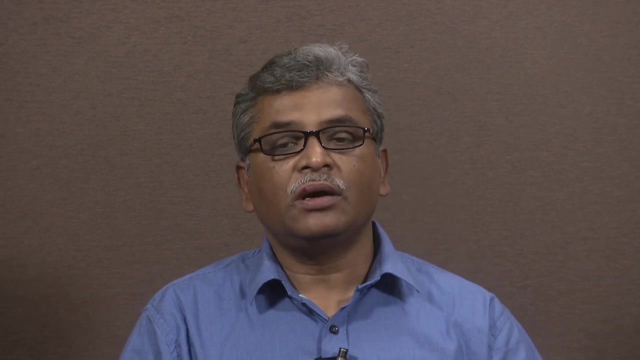 as well as specific cake resistance from the experimental data, just by taking that volume of filtrate with respect to time, Also there it is discussed that what are the- you know- basic modes of that operation? either it will be constant rate filtration, or it will be filtration or constant pressure filtration or not. So there we have discussed both the. 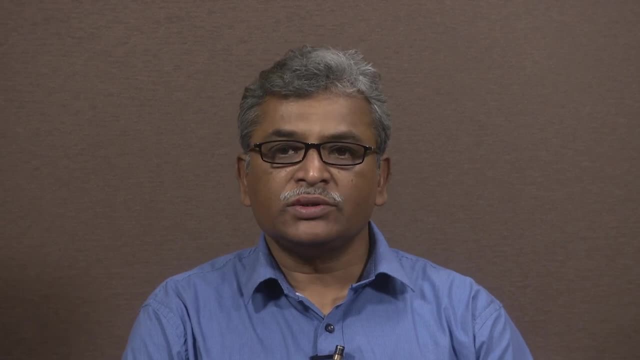 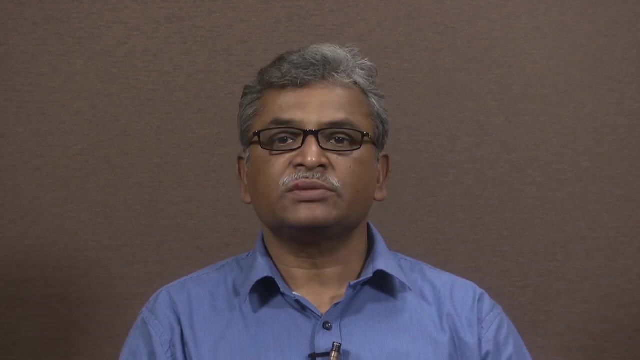 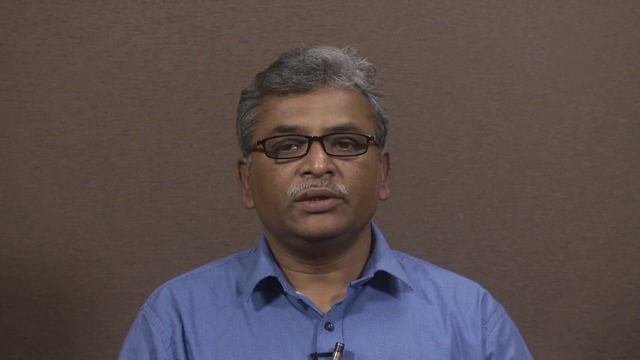 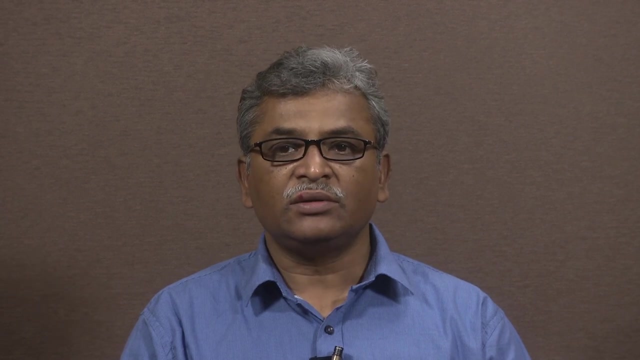 modes there. Today's lecture will be including also that regarding the filtration, but it will be different mechanism. it is called that, you know, reverse osmosis process. Here also, the filtration process will be governed by the, you know, driving force of pressure And in this case some terms should be there that will be discussed and also what will 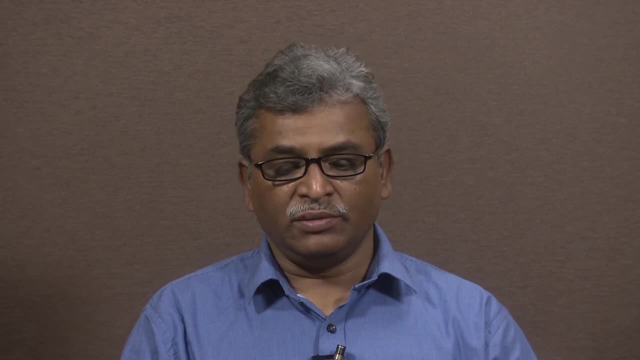 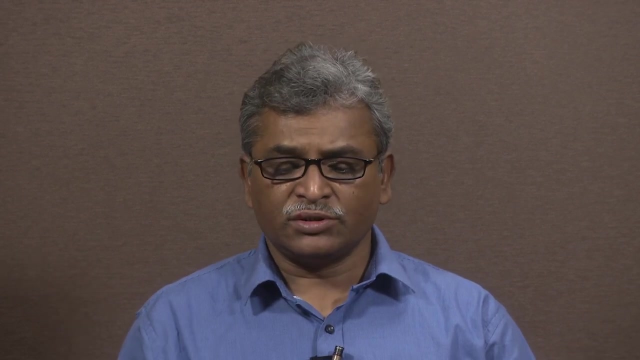 be the mechanism and how to assess this. you know reverse osmosis process, where it can be applied and also what is the basic mass transfer equation for assessing this reverse osmosis. it will be discussed here. So before going to that reverse osmosis, you have to 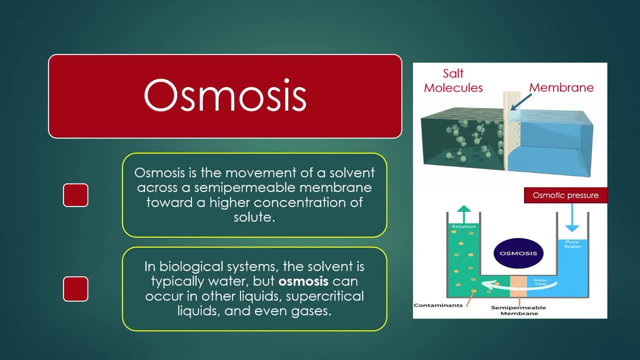 know what is osmosis. So what is osmosis? basically, it is the movement of, you know, solvent across a sample semipermeable membrane towards a higher concentration of solute. Suppose there is a solute. here in this picture it is shown that if suppose there is a solution of having some solute, 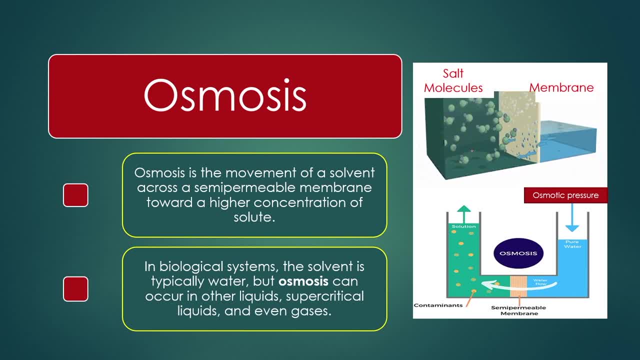 and there will be a certain concentration of that, you know solute here in this solution, whereas in the opposite side of a membrane which is placed here between these two, you know solution here, other side of this membrane, there will be no solute. So here pure solvent. 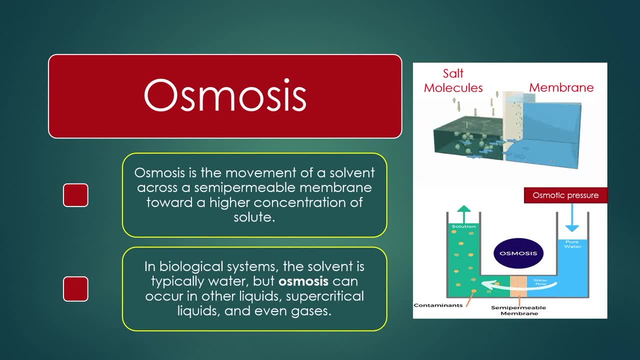 you can say So. you will see that there will be a movement of solvent across the semipermeable membrane towards a higher concentration of the solute. So where that concentration? here you will see that the concentration of that solute will be higher relative to the concentration. 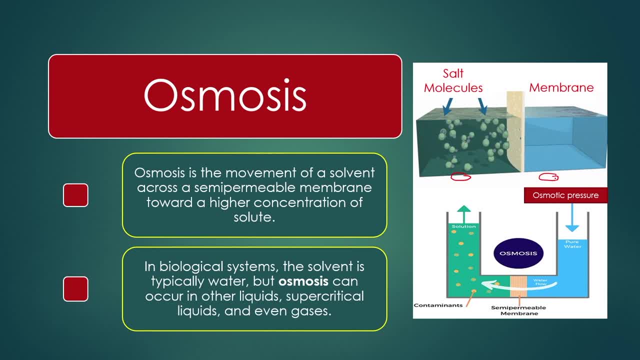 of the solute here. If here there is no solute, then it will be concentration 0, whereas there will be certain amount of solute. The solution here is a captened in the presence solute in the solution. So we can say that this go be higher. you know concentrated solution, and here this is. 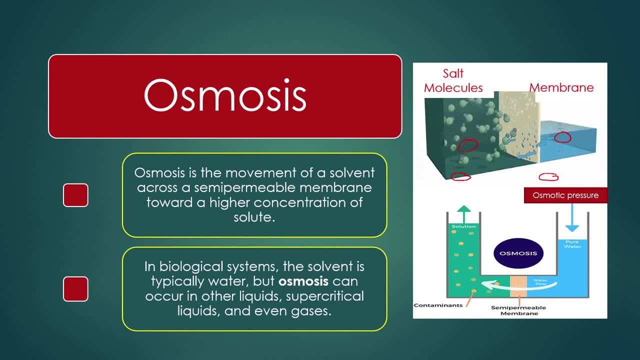 the, you know, pure solvent, there will be no solute. So there will be a movement of this, you know solvent, from this to know lower concentration to the higher concentration solution. So this actually mechanism of movement, or this transport of this, the solvent, from its lower 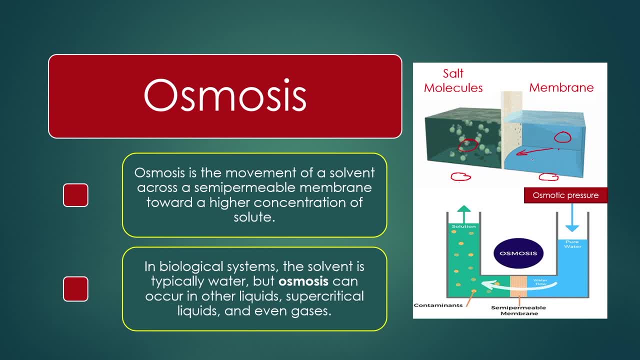 lower concentration to the higher concentration will be regarded as that osmosis. okay, In biological systems you will see that solvent is typically water, but osmosis can occur in other liquids, like you know, supercritical liquids and even gases. also there you can. 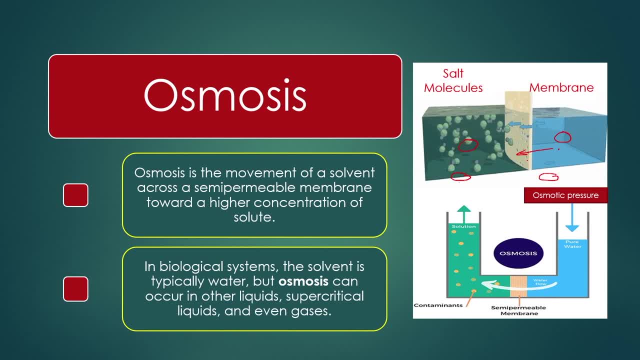 say that means gases will be moving from lower concentration to the higher concentration. So this is called osmosis. This is the basic you know concept of this osmosis: osmotic pressure by which that solvent would be moving from the lower concentration to the higher. 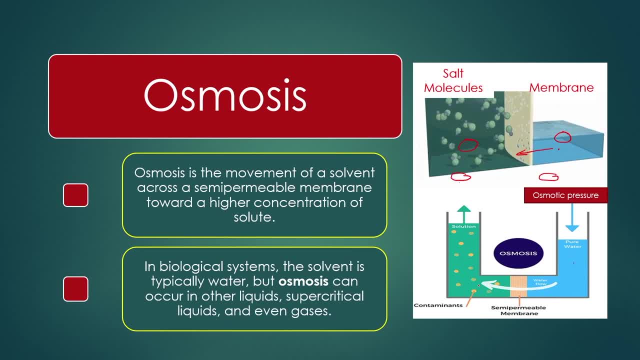 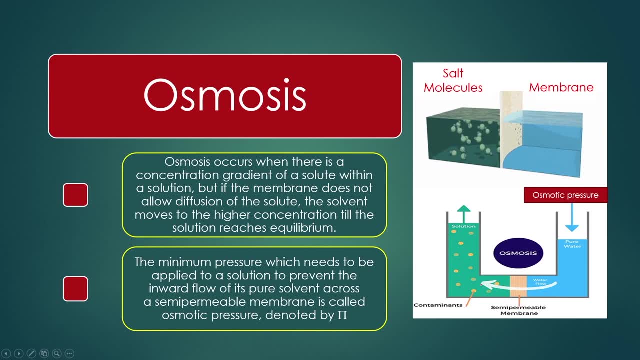 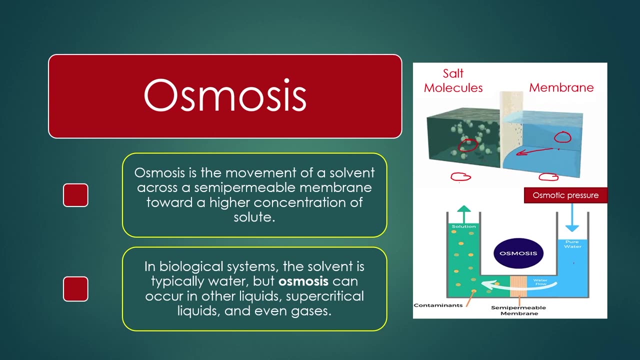 concentration. So here the osmotic pressure is the driving force. okay, So this is called osmosis, Whereas you will see that reverse osmosis what There? the direction of the movement of the solvent will be opposite because of that applying some pressure externally. So 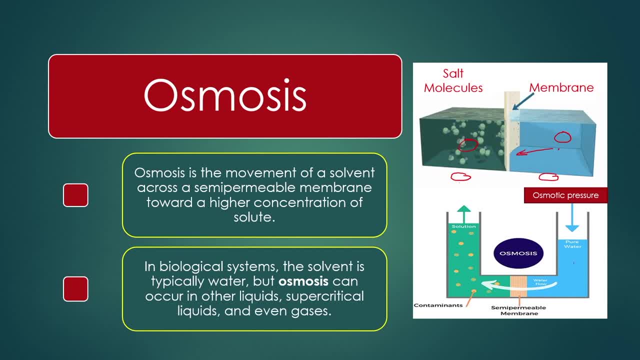 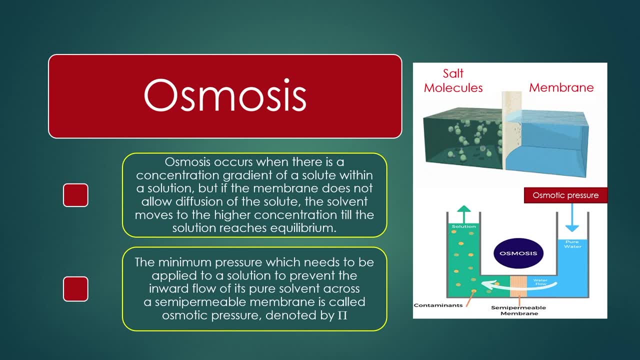 that will be a reverse osmosis. So that will come later. So let us go to the next slide. So let us discuss about this osmosis again here. So osmosis will occur when there is a concentration gradient of solute within a solution, but if the membrane does not allow. 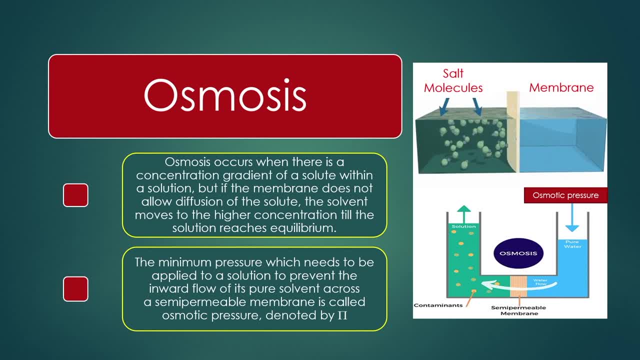 diffusion of the solute. the solvent moves to the higher concentration till the solution reaches equilibrium. So here the solvent will move up to when The solvent will be moving till this, you know, concentration of this higher concentration, that till the solution reaches its equilibrium. 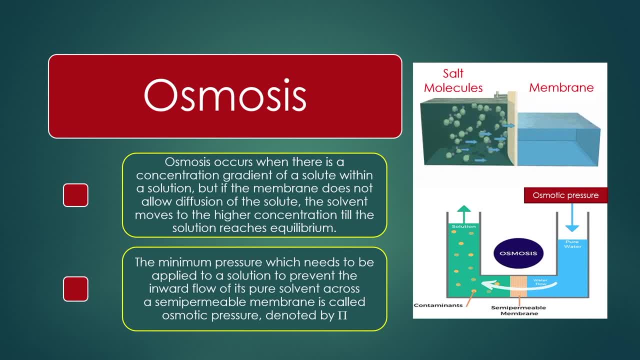 That means, in the both the cases you will see that there will be a equilibrium condition. okay, So in this case you know that there will be a concentration gradient of a solute within a solution, but if the membrane does not allow diffusion of that solute, the solvent moves. 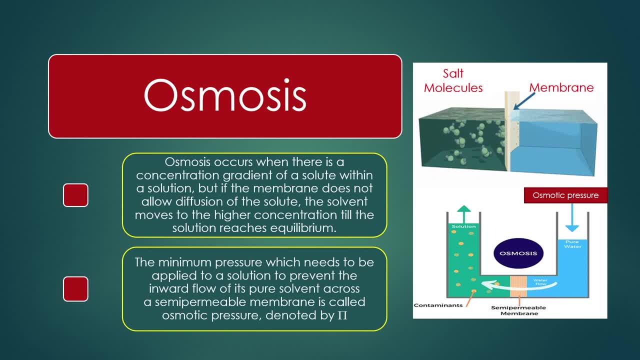 to the higher concentration till the solution reaches its equilibrium. Now let us discuss about this osmosis. So this is the osmosis. So this is the osmosis Now, the minimum pressure which needs to be applied to a solution to prevent the inward 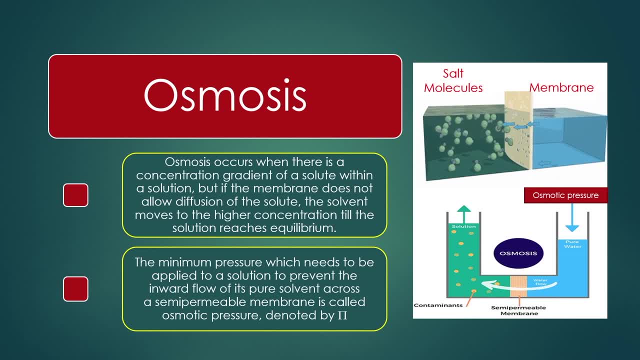 flow of its pure solvent across this semi-permeable membrane is called that osmotic pressure. So by osmotic pressure this pure solvent will be moving to that higher concentration. So it is denoted by phi, So phi is called osmotic pressure. In earlier lecture we have also 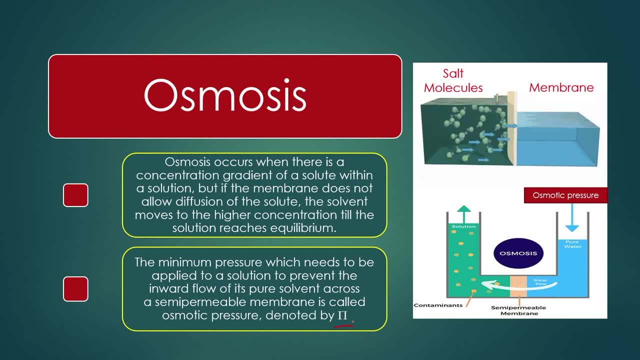 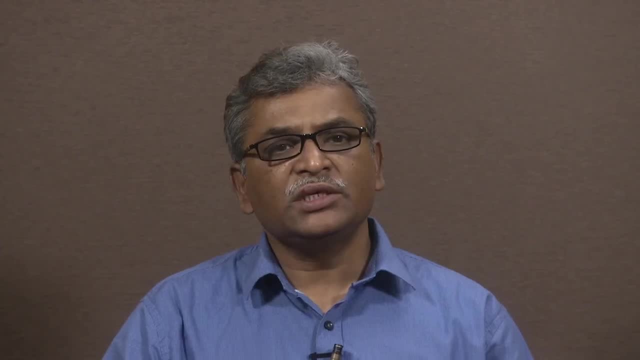 shown that there will be a net pressure based on which that filtration happens. That net pressure is the total pressure minus that osmotic pressure. But when we are talking or we are actually doing the operation with the pure solvent, in that case this osmotic 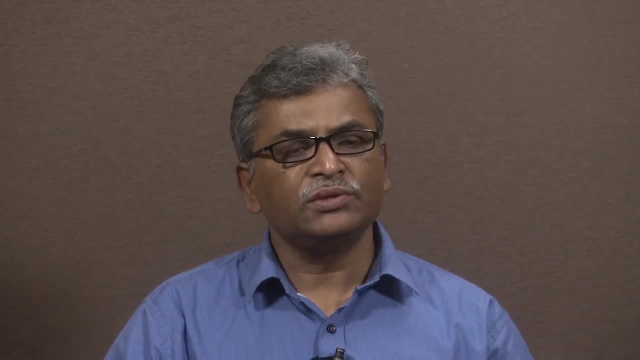 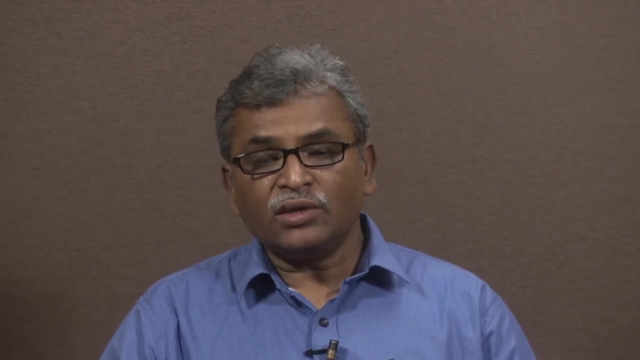 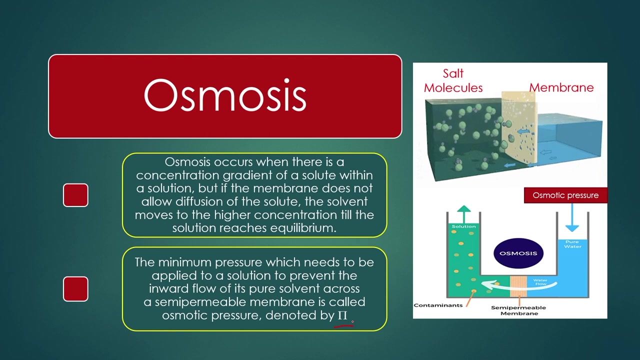 pressure will be very negligible compared to the total pressure. So in that case phi is considered as a negligible amount. So there it is neglected, But here osmosis. So you, In that case it is the natural process. you can say that solvent will be passing from. 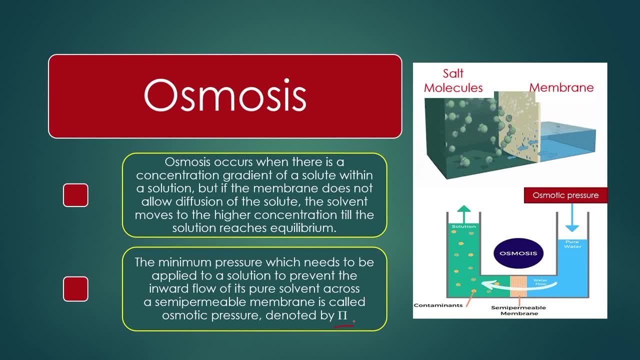 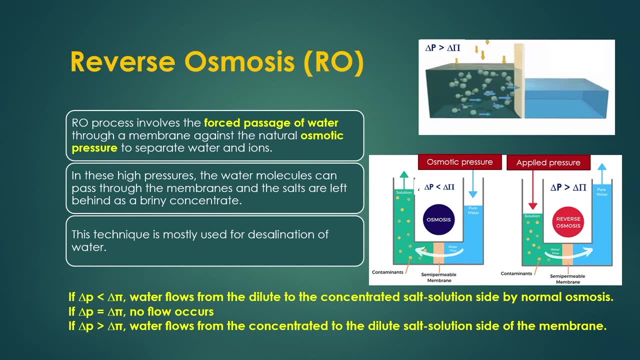 this lower concentration to the higher concentration by this pressure- This is called osmotic pressure- And then reverse osmosis. coming Now, in this case you will see that in this figure the higher concentrated solute will be that tend to be applied to this high pressure. 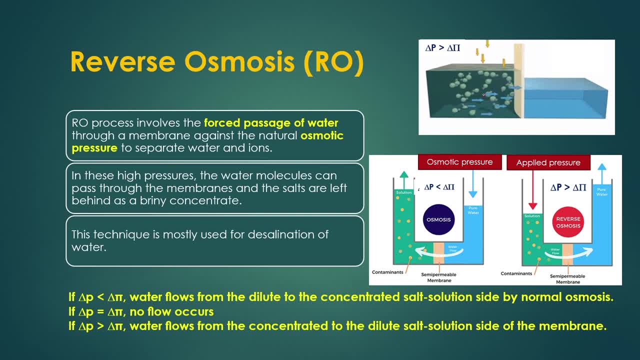 Because of this high pressure, you will see that the solute particles will not be passed through that membrane, whereas the liquid or solvent will be passed through that membrane because of that high applied pressure. So in this case movement of that solvent will be in the reverse direction. 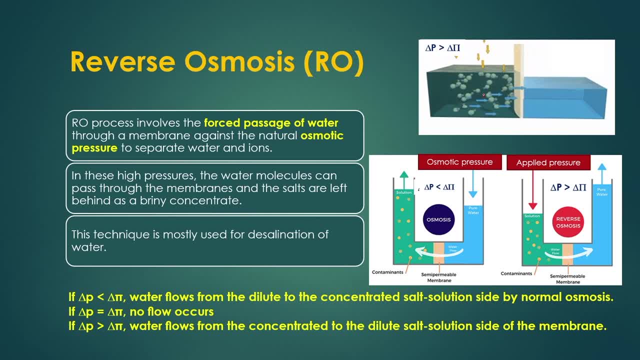 In this case the solvent from the higher concentration to the lower concentration will be moving, So it will be basically under a pressure which will be greater than that osmotic pressure. So the RO process involves. RO means reverse osmosis. this is a short form. 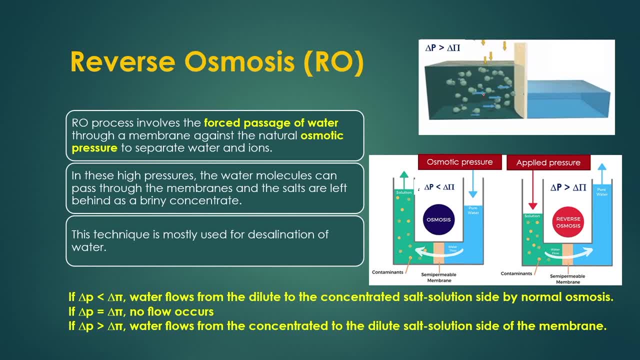 So RO process involves the forced passage of water or solvent through a membrane against the natural osmotic pressure to separate water and some solute. Solute may be ions or other things. In these high pressures greater than that osmotic pressure, The water molecules can pass through the membranes and the salt are left behind as a briny concentrate. 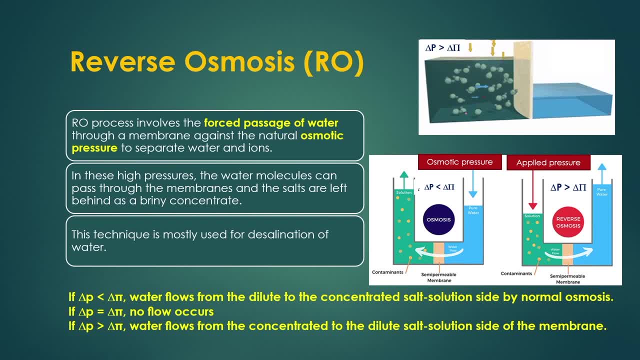 So that means here we will see that in this amination process we will see that from this higher concentrated solution of that solute the solvent will be passing through that membrane, whereas solute remains or it will be separated by this membrane there. 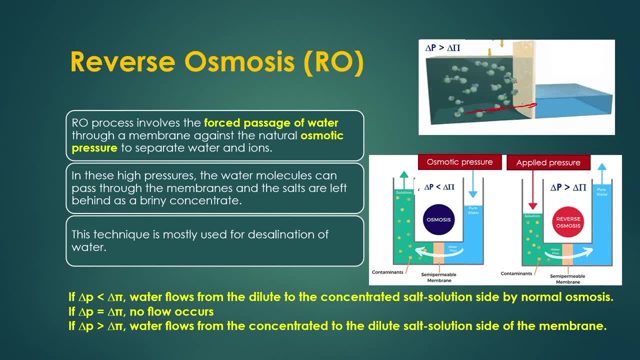 That means solute will not be passing through that membrane. So this takes place. So this technique is mostly used for desalination of water, Especially you will see that when we are actually making drinking water from the sea water. So in that case this reverse osmosis is very important. 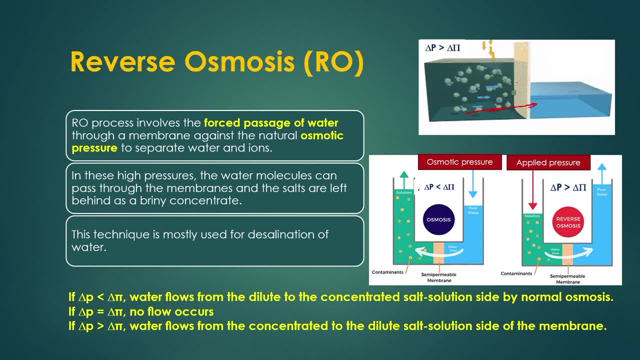 And in large scale industrial operation it is being done that reverse osmosis, whereas in our domestic use also there are some systems that is called reverse osmosis systems also available And they are also used. There are also some solid particles to be separated by this reverse osmosis mechanism. 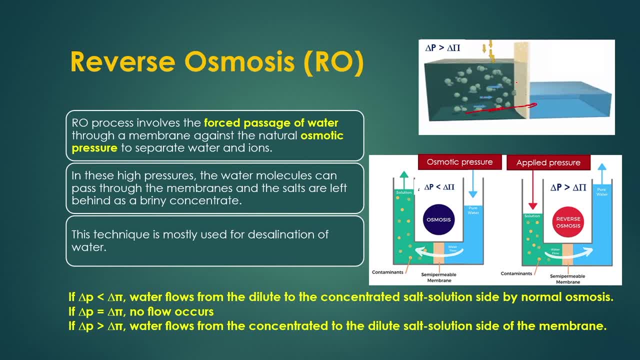 So in that case there will be a certain membrane through which that solute will be retained under this high pressure, just by allowing the clean water there. So if delta P- that means applied pressure- is less than delta Y, that means osmotic pressure, 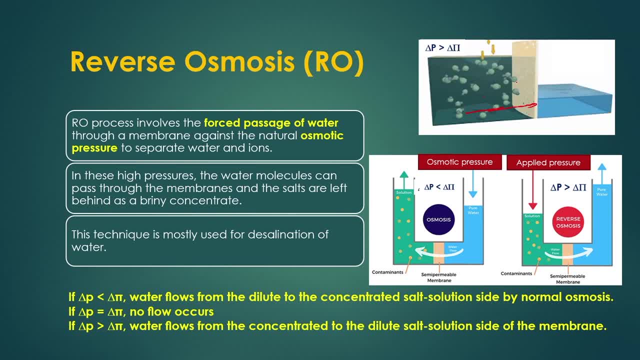 then water flows from the dilute to the concentrated solute. So if delta P, that means applied pressure, is less than delta Y, that means osmotic pressure, then water flows from the dilute to the concentrated solute- Here also the washer solution side- by normal osmosis. 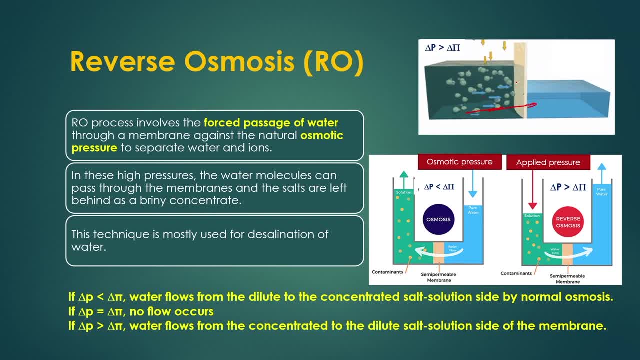 And if delta P is equal to delta Y, so there will be no flow occurs. That means equilibrium condition would be there. If delta P is greater than delta Phi, then water flows from the concentrated solution to the dilute salt solution side of the membrane. 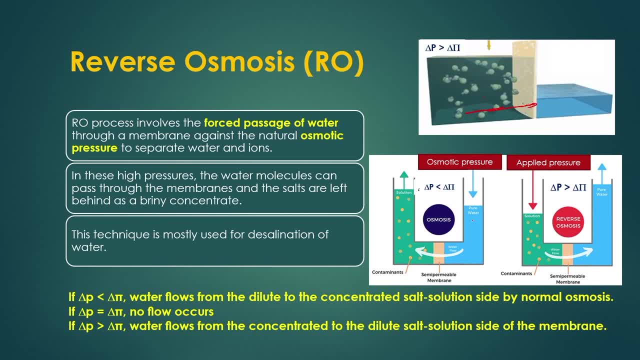 Here in this picture also, it is shown that under this osmotic pressure we will get a micro beverage, in this case. Okay pressure. this solvent is flowing from this, you know, lower concentration to the higher concentration, where, in the reverse osmosis, the solvent will be flowing from the higher. 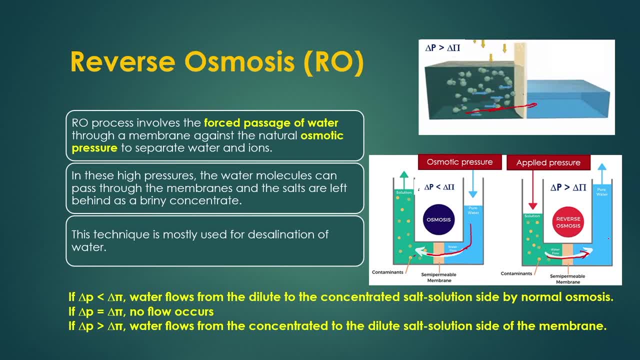 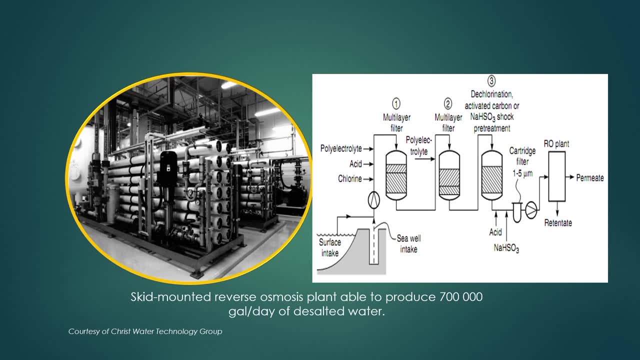 concentrated solution to the, you know, lower concentrated solution through the semipermeable membrane. Then in industrial scale you will see that Christ water technology group. they are producing drinking water commercially in a large scale. that is, capacity is very high. In that case they are separating different solute by this reverse osmosis technique. 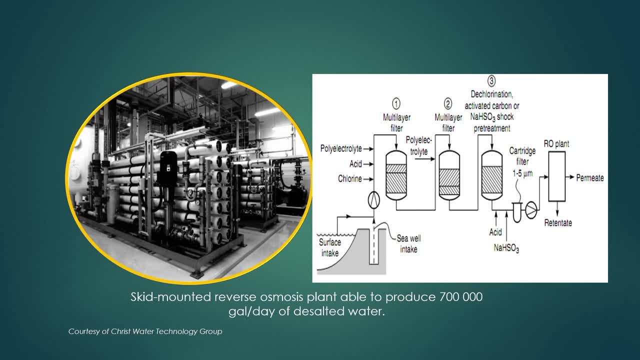 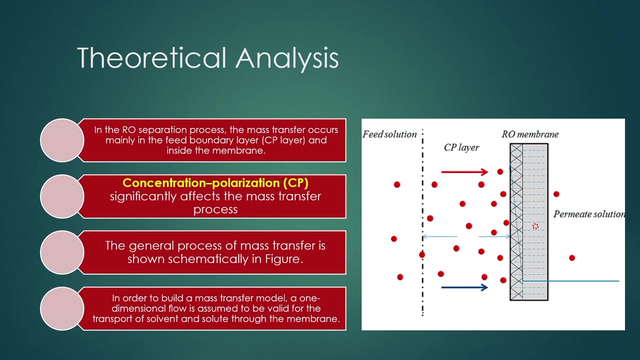 And they are producing this. you know potable water, that is, desalted drinkable water around. you know that 7 lakhs gallon per day from this. you know that salting water. Now we will assess this reverse osmosis technique, which is actually governed by that driving. 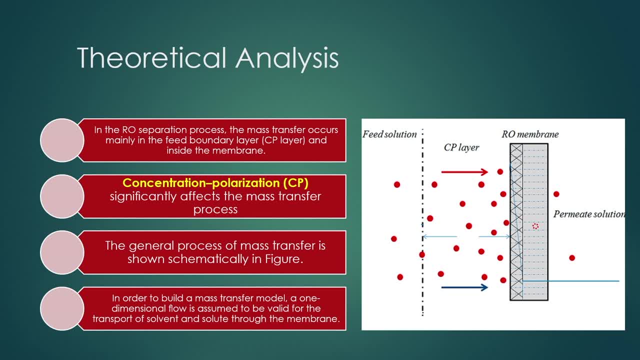 force of pressure drop and how to assess, how to assess this? you know, reverse osmosis separation process. There will be a certain. you know, mass transfer happens mainly in the feed boundary layer and the inside, The membrane. what is that feed boundary layer and also the whatever mass transfer. mass transfer. 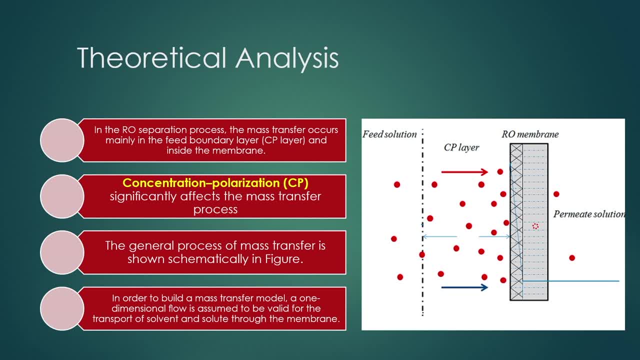 means here solute transfer, here from one concentrated solution to the another. you know diluted solution, So there will be transport of that solute. it is called mass transfer. So here some boundary layer of the solid particles near about that membrane. you will see that that will affect. 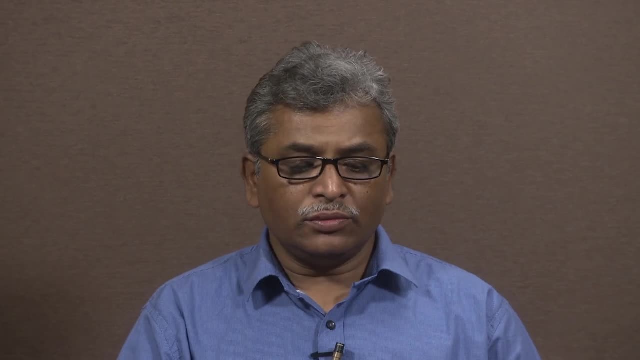 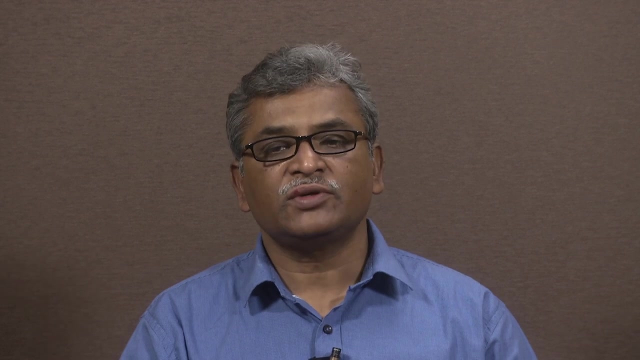 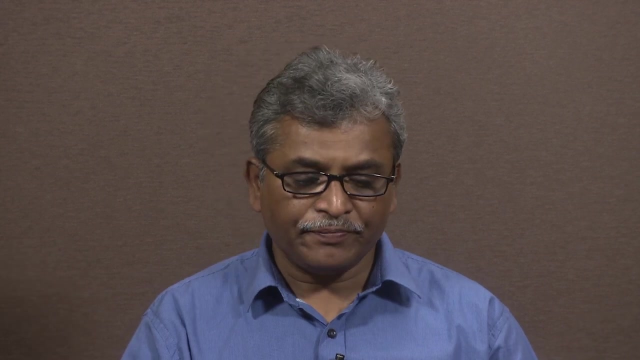 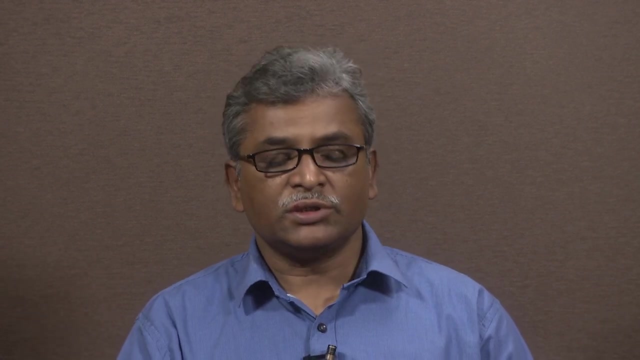 That you know mass transfer and also you will see that some operational process variables also will affect that. you know mass transport of solute from high concentrated solution to the dilute solution through the- you know- membrane, under that pressure, And now in that case that mass transfer model to be used to assess that you know reverse. 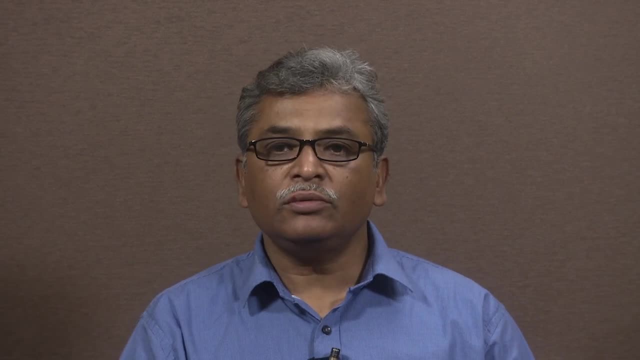 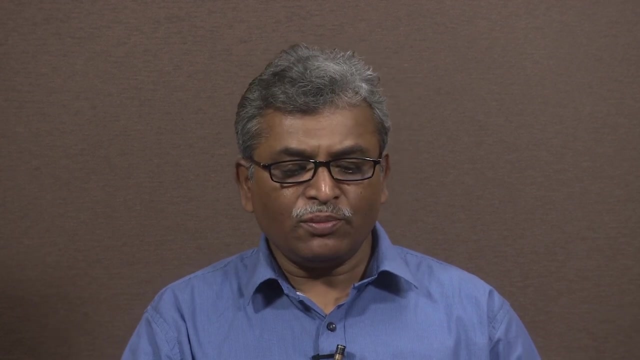 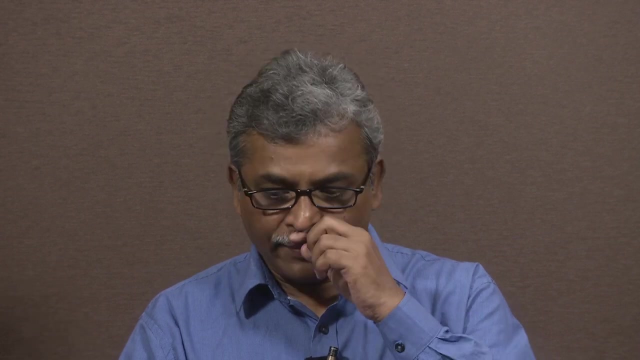 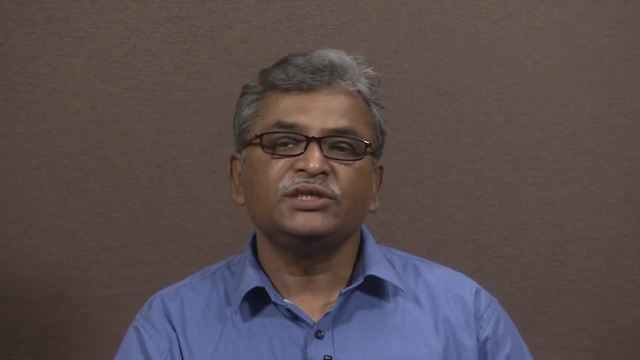 osmosis separation process. For that you have to know some. you know Concept of concentration polarization. what is that concentration polarization? here you will see that some particulate materials or solute, you can say here the concentration layer will be different along the distance in the bulk region of that. you know solution. 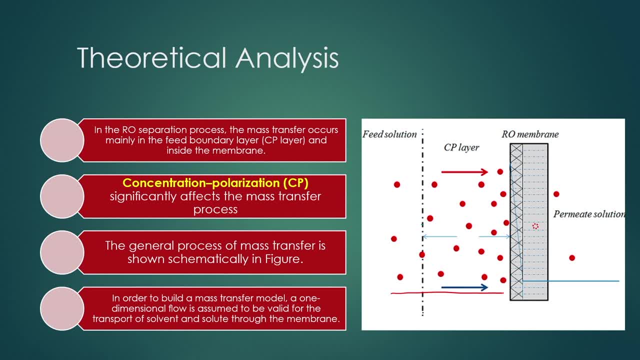 highly concentrated solution. suppose this solution is the concentrated solution and this is the membrane, And In this side of this membrane The concentrated solution is there and the other side of the membrane to be, you know, dilute solution, that means the concentration of that solute will be very low, whereas clear. 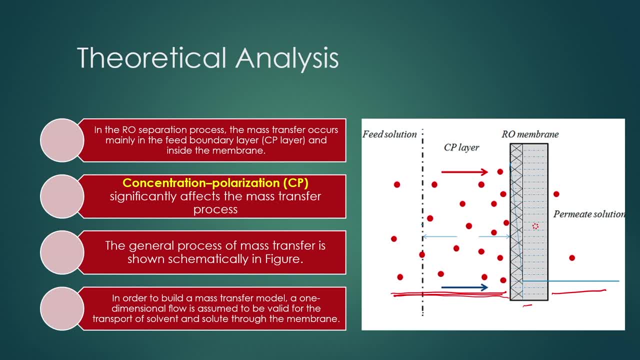 liquid, you can say that it will be passed through that membrane. So in this side, where concentration of that solution, you will see that particle concentration it will be different at a different location. Where that feed solution Is Entering The entry zone, you will see that the concentration of the particles or solute will be. you know. 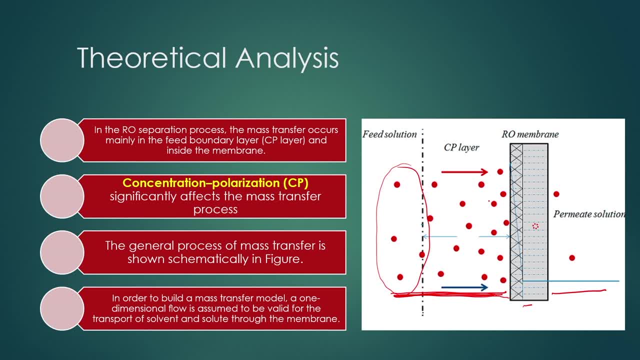 very low compared to the region which is adjacent to that membrane. So in that case where that solute concentration will be relatively, you know, higher at that, adjacent layer of that, you know adjacent, you know side of that, you know membrane. So in that case where that solute concentration will be relatively you know higher at that. 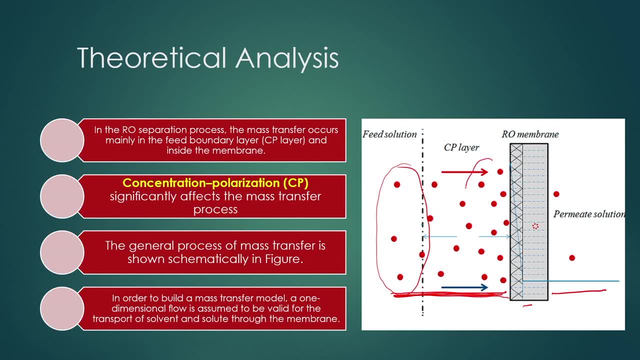 membrane. There the concentration will be higher. So this will be regarded as a concentration polarization layer. that means solute will be polarized to be coming to this side of this membrane and when, with respect to time, it would be coming and depositing in this side of this membrane, it will be deposited. 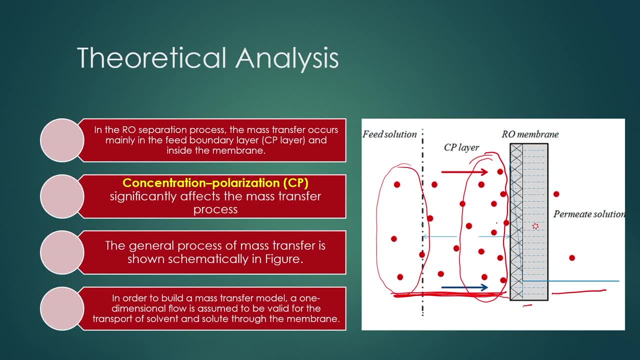 as a layer. So that is why concentration of the particles will be higher in this side. So it will be. So this particular zone it will be, you know, regarded as, or will be defined as, a concentration polarization layer or concentration polarization zone. So, in order to build a mass transfer model, you will see that a one dimensional flow to 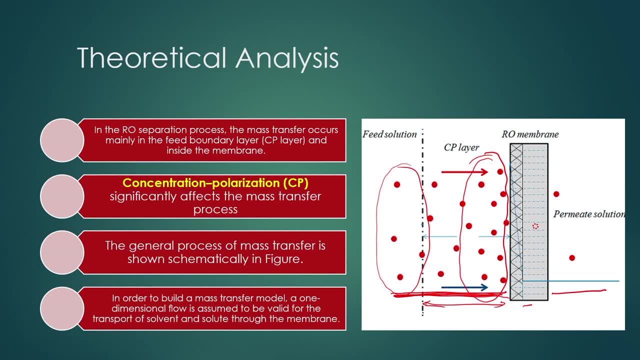 be assumed, which is to be valid for the transport of this solvent and solute through the membrane. So for that you have to know the concentration of the particles. So for that you have to know the concentration of the particles. So for that you have to know the concentration of that solute. in this concentration, polarization. 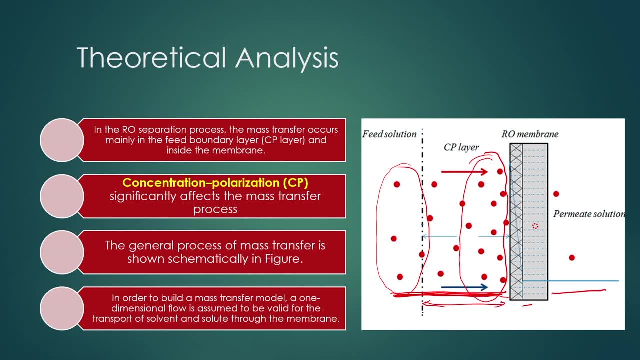 region. So whenever you are going to assess that mass transfer of that solute to this membrane, you have to know that concentration difference of this solute, either in this you know concentration polarization region or in the permeate region, in the permeate solution. Now, on the basis of that concentration polarization, 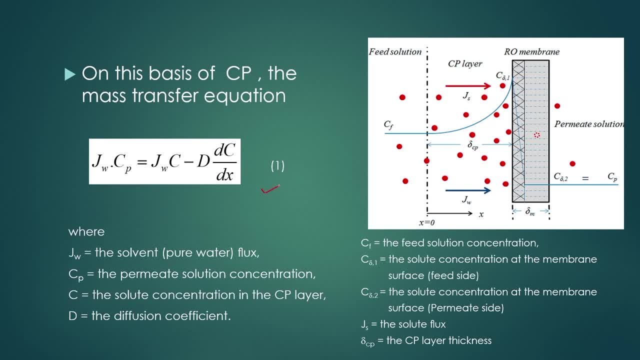 The mass transfer equation can be written based on the, you know, mass balance equation by this equation 1, where you will see that Jw Cp, that will be equal to Jw C minus d, into dc by dx, where Jw is the solvent. you know flux, flux, you know that that means rate of. 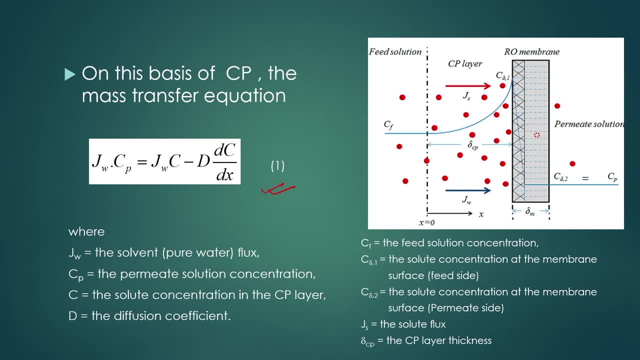 volumetric flow, Right The flow of that solvent per unit cross sectional area of the membrane. that is called flux and here Cp. Cp is basically the permeate solution, concentration, and C is called the solute concentration in the concentration polarization layer, Here Cp, as shown in the picture here. what is the Cp concentration? here Cp is, C is the. 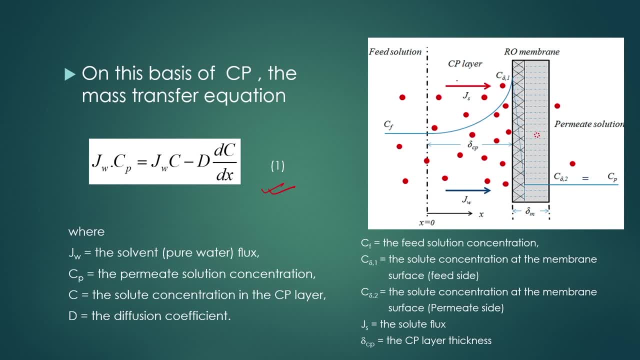 solute concentration in the- you know, Cp layer. here in this region, C, Right And D is the diffusion coefficient. So here in this case we can say that there will be a certain concentration gradient with respect to x in this concentration polarization region and this concentration, you know, gradient. 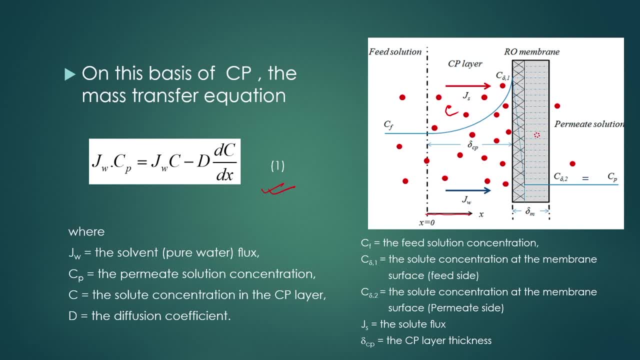 with respect to x, in this direction of flow. this will give you the diffusion. what amount of diffusion will be there? Rate of diffusion, you can say So this will be basically minus d, dc by dx, where d is a diffusion coefficient as per fixed law of diffusion. and then what will be the other flow of that? you know, solute. 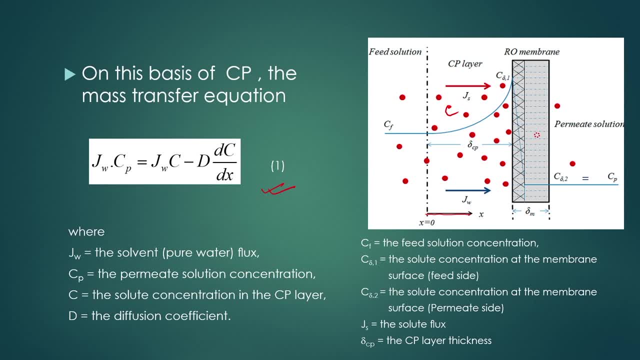 that will depend on that. you know solvent flux. So in that case, what will be? the solute will be transported by that solvent flux, this will be Jw into C, whereas by diffusion. how that solute also to be transported, that will be minus d dc by dx. 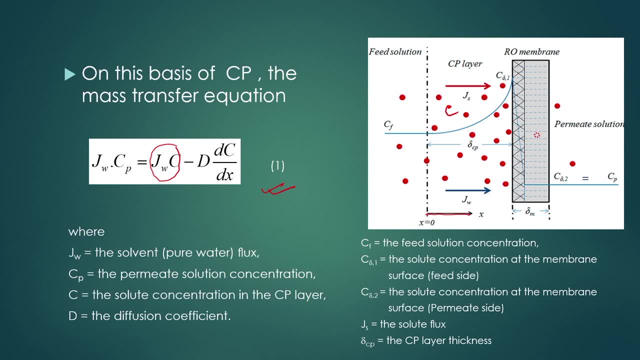 So what is the effective? you know that transport of that solute. that will be regarded by this Jwc minus d, dc by dx. So that will be basically what is the Jw into Cp. this is what is that? the amount of solute, solute. 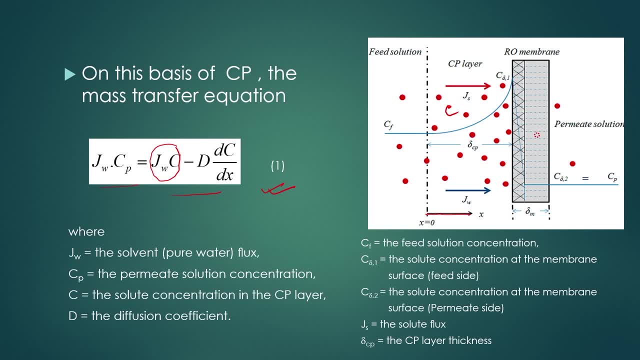 Which is actually transported through the membrane at that particular solvent flux. okay, and in this representation of this schematic diagram, you will see that there it is written Cf. Cf is basically the feed solution concentration. C delta 1 is term. this is basically the solute concentration at the membrane surface. this is C delta 1 and C delta 2. you will see that. 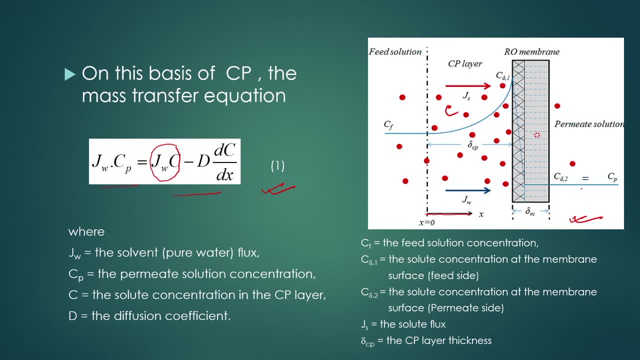 it is the solute concentration at the membrane surface that is in the permeate side, And another terms. you will see that there will be Js. Js is basically the solute flux and delta Cp is called the length of that Cp layer or thickness of that Cp layer concentration. 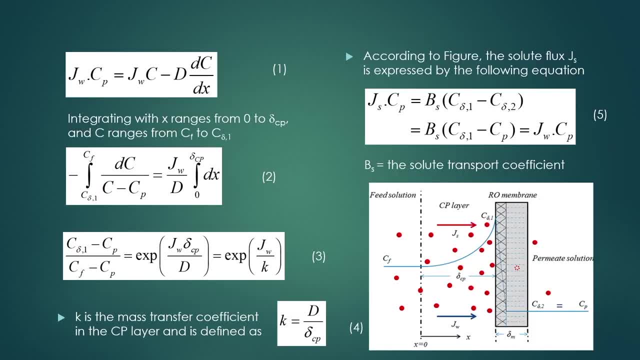 polarization layer. So we are having that, you know, mass balance equation. That is represented by equation number 1, that is Jwcp. that will be Jwc minus d, dc by dx. Now, if you do the integration within a certain boundary condition, that means x is ranges. 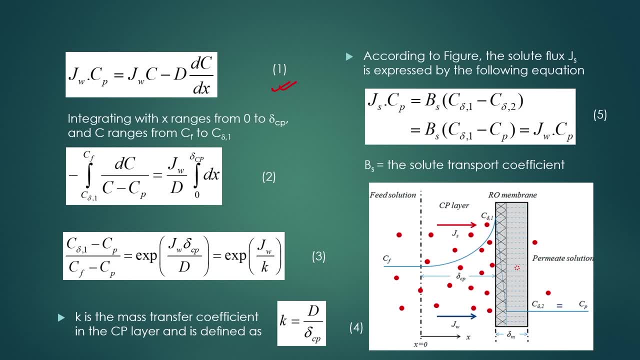 from 0 to delta Cp and concentration will be ranging from C1 to C delta 1. within that, you know, x ranges. So, based on this boundary condition, So we can integrate this equation number 1 and then we can get this equation number 3 as C delta 1 minus Cp by Cf minus Cp, that will be equal to exponent of Jw delta Cp by. 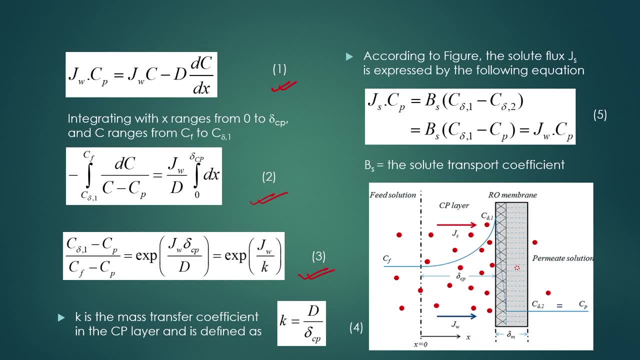 d is equal to exponent of Jw by k. So this equation number 3 will give, after integration of this equation number 1, with that boundary condition, And this equation will be called as that, you know, governing equation for this reverse osmosis filtration process. 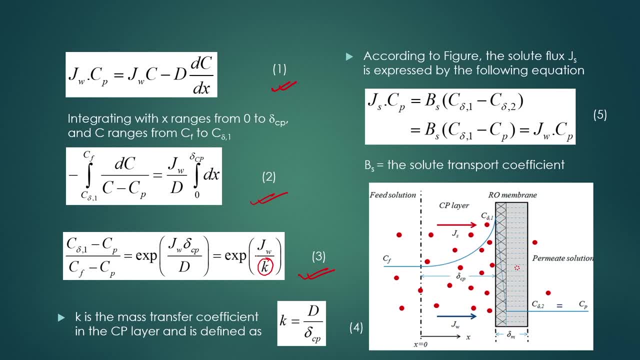 In this case one term. you will get this: k. k is basically the mass transfer coefficient in the concentration polarization layer and is defined as k will be is equal to d by delta Cp. So d is called diffusion coefficient And delta Cp is called diffusion coefficient. 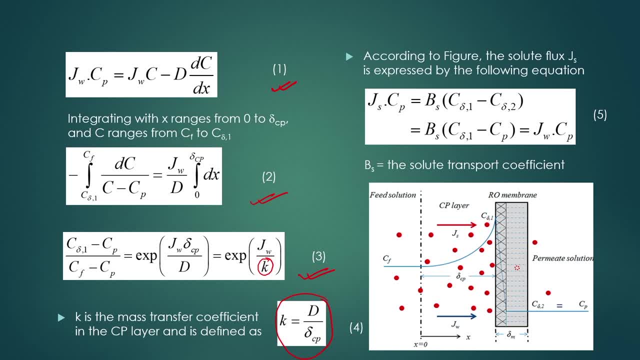 And delta Cp is called diffusion coefficient. So this equation number 3 will give, after integration of this equation number 1, with that thickness of that boundary layer, of that concentration, polarization. Now, according to this figure, you will see that the solute flux Js is expressed by the 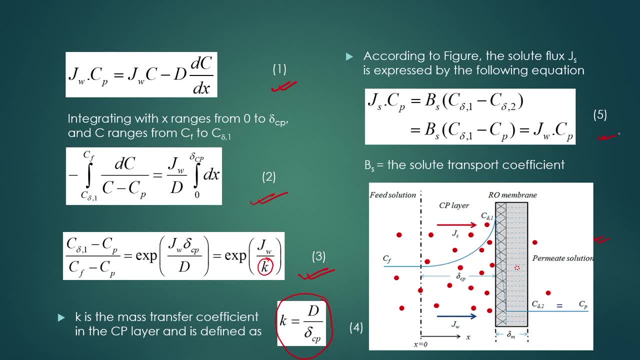 following equation: This is fine because it is coming from that you know concentration differences. So it will be basically: Js into Cp, that will be: is equal to Vs And this is the concentration. So this is the concentration: Vs into C delta 1 minus C delta 2.. 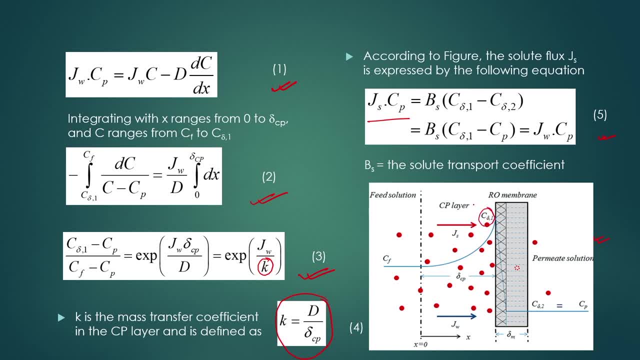 Here this is C delta 1, the concentration of this solute in the- what is that retentate side of the membrane, whereas C delta 2 is the concentration of solute in the permeate side of that membrane. So this concentration difference will give you the expression for the mass transfer of. 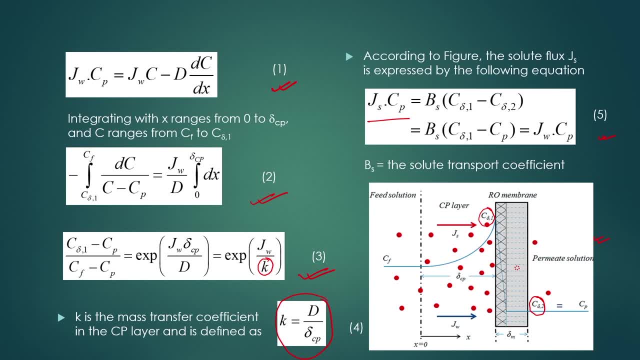 that solute, okay, which can be represented by this equation, number 5.. Also, it can be expressed by the concentration difference of this you know C, delta 1 and this you know Cp. Cp is basically what is that concentration of solute in the permeate solution which will 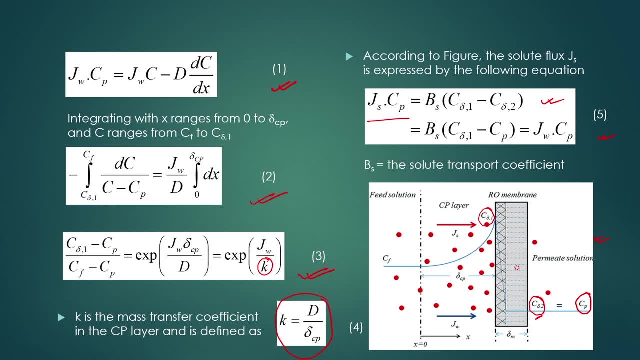 be exactly the same concentration in the near region of that. you know Cp. Okay, Thank you, Thank you. Thank you. You know membrane at this permeate side, So we can write this equation, number 5, according to this figure based on the concentration. 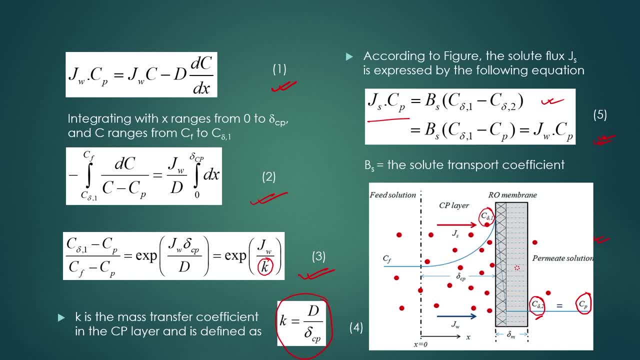 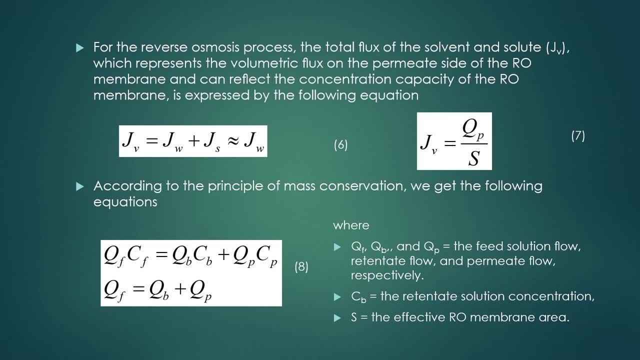 difference for this mass transfer equation, where Vs is called solute transport coefficient, Now for the reverse osmosis, so the total flux of the solvent and solute, which represents the volumetric flux on the permeate side of the reverse osmosis membrane and can reflect 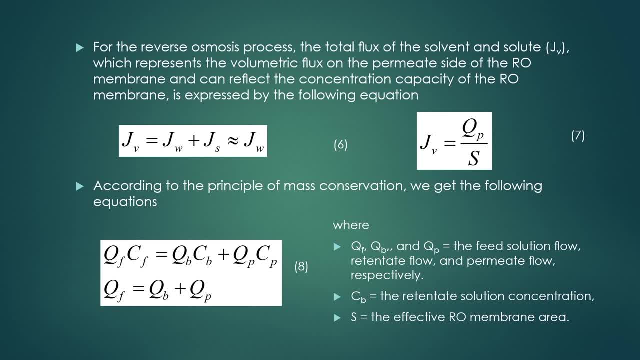 the concentration capacity of the reverse osmosis membrane, which can be expressed by the following equation: here equation number 6.. Here Jv. Jv is basically the total flux of the solvent and solute, which is basically Jw plus Js. and since Js is very negligible compared to that Jw, then Jv can be regarded. 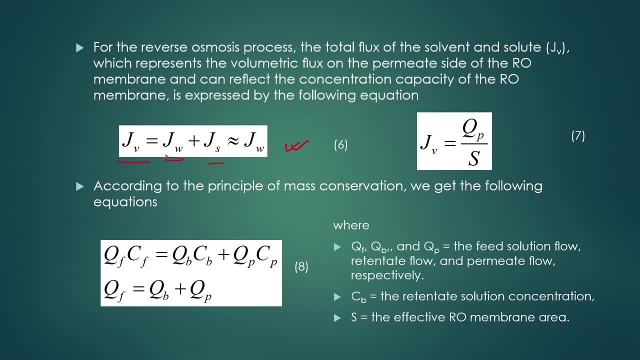 as Jw here itself, Where Jv can be defined by this volumetric flow rate divided by the surface area of that membrane through which that feed will be flowing or solute will be releasing Okay, Okay, Okay, Okay. retentate or solvent will be transporting. Now, according to that principle of mass conservation, 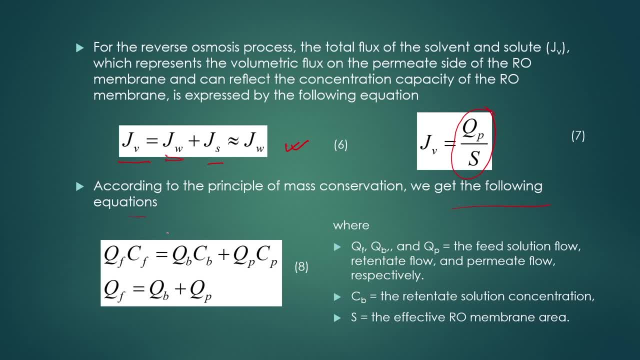 we get the following equation: here we can write that mass conservation equation: what is the total solute that is in feed that will be is equal to what QB into CB plus QP into CP. that will be is equal to QB means what that means here, the you can say that feed. 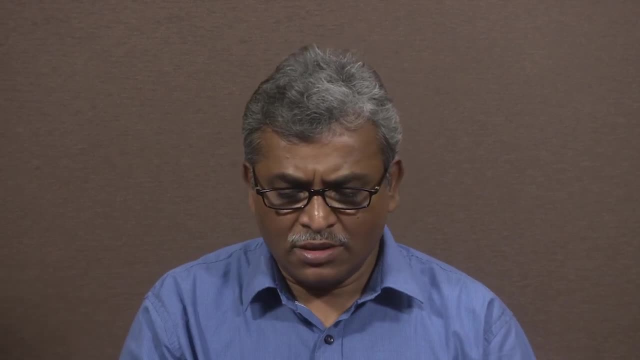 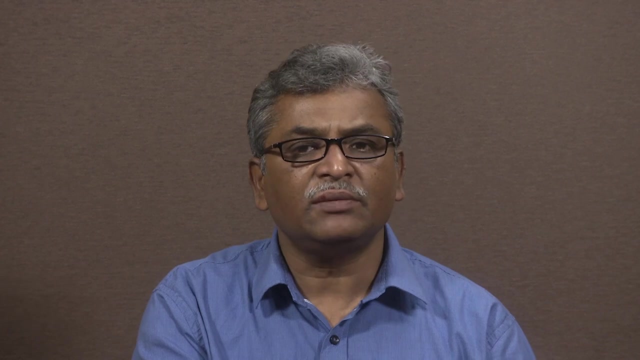 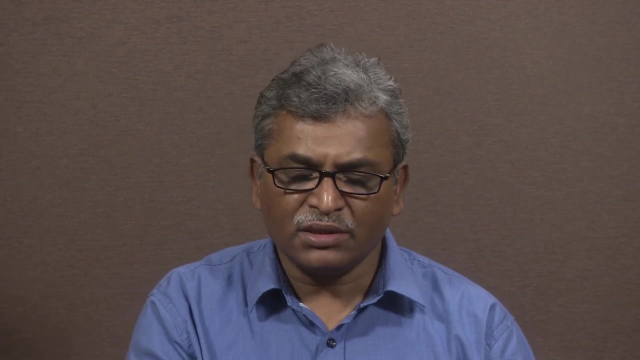 no, here it is basically that retentate flow rate. retentate flow rate, you can say: and CB is the concentration at that. you know, retentate flow, that means at the bulk flow. you can say: and CP is the concentration of solute in the permeation solution or permeate solution. 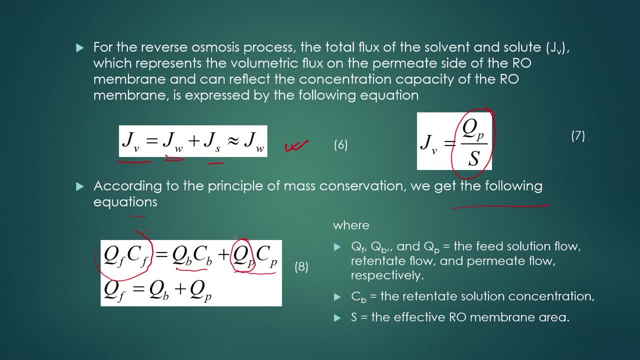 and QP is the permeate flow rate. So QF, QB and QP, these are actually feed, solution flow, retentate flow and permeate flow respectively. and CF, CB and CP are the solute concentration respectively. Also, the total balance of that solute can be, you know, regarded as QF. that 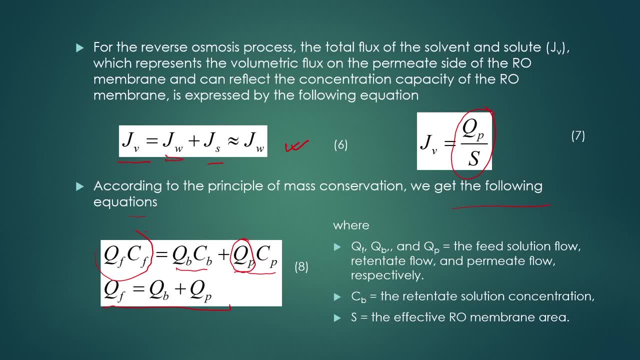 will be is equal to QB plus QP. So here QF is basically solute and solvent, QB also solute and solvent, QP also solute and solvent in the feed bulks, or retentate, you can say, and also permeate side of that. 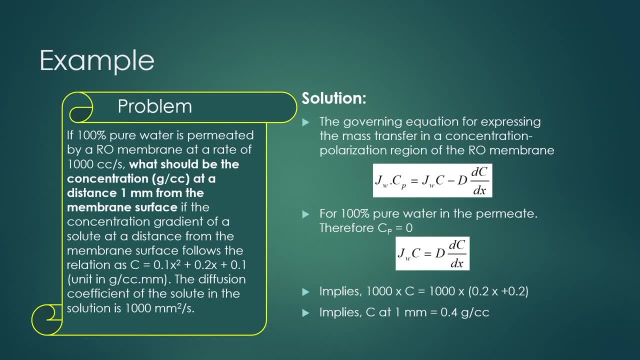 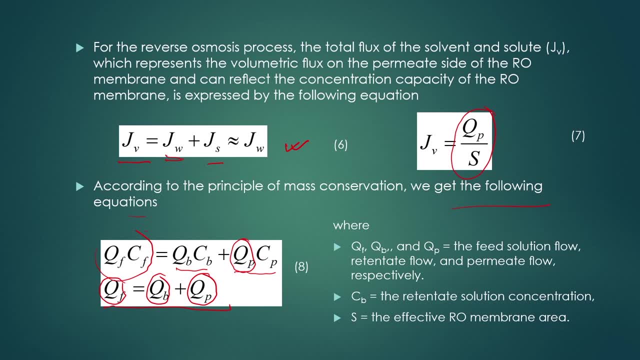 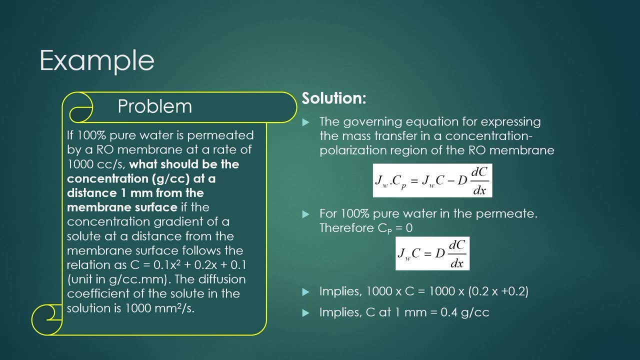 membrane. And so this is actually the you know governing equation to, you know, assess this, you know membrane separation process by this reverse osmosis. Now let us do an example based on this you know theory. Suppose 100 percent pure water is, if permitted, by a reverse osmosis membrane, at a rate of 1000 cc per second. what should? 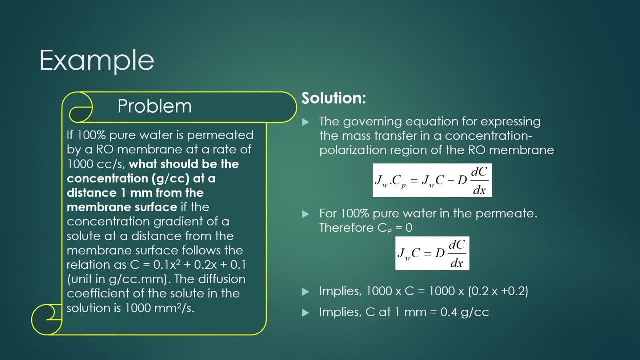 be the concentration, that is, per gram per cc at a distance 1 millimeter from the membrane surface. So if the concentration gradient of a solute at a distance from the membrane surface follows the relation, as C will be, is equal to 0.1 x square plus 0.2 x plus 0.1, where unit is. 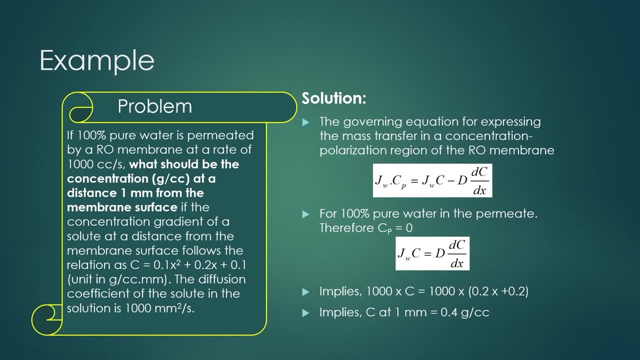 given in gram per cc per millimeter. The diffusion coefficient of the solute in the solution is given 1000 millimeter square per second. So for this problem you have to find the gradient of mass G. So what you have to find 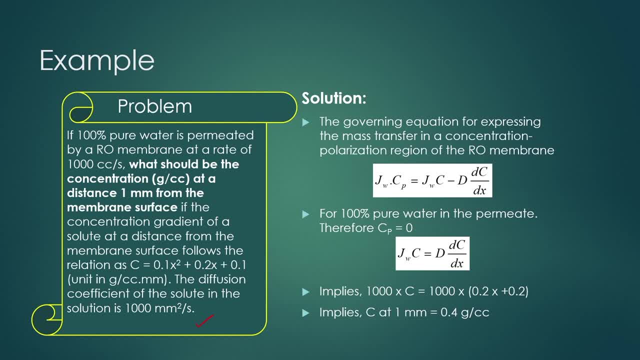 out. you have to find out what would be the concentration at a distance 1, millimeter from the membrane surface. You have to find out what is the C value, The governing equation for expressing the mass transfer in a concentration polarisation region of the RO membrane which. 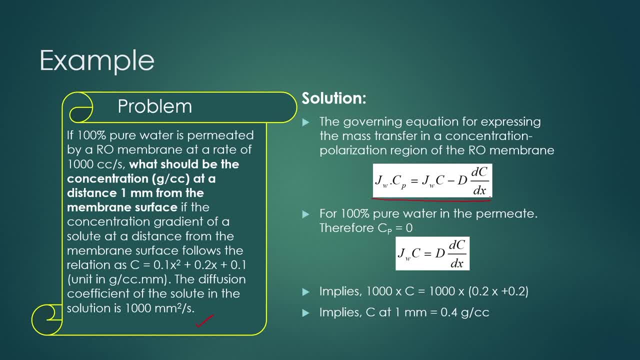 can be retained by this equation Here: j WCP. that will be equal to j Wc minus D dC by df For 100% pure water in the permeate. in that case we can write that Cp will be is equal to 0,. since 100% pure water, there will be no solute there. so Cp will be is equal to. 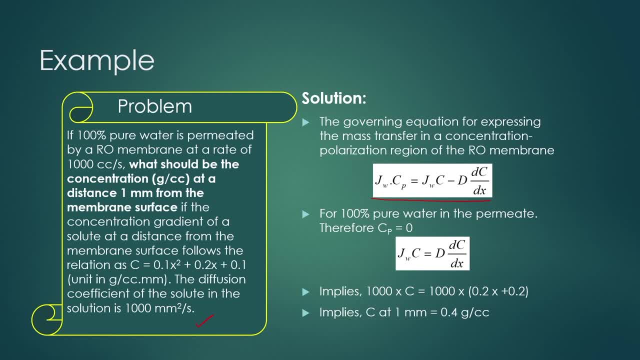 0. So we can write Jwc that will be: is equal to d into dc by dx. from this equation, which implies that Jw is given 1000, see, we have to find out d again 1000 into dc by dx it. 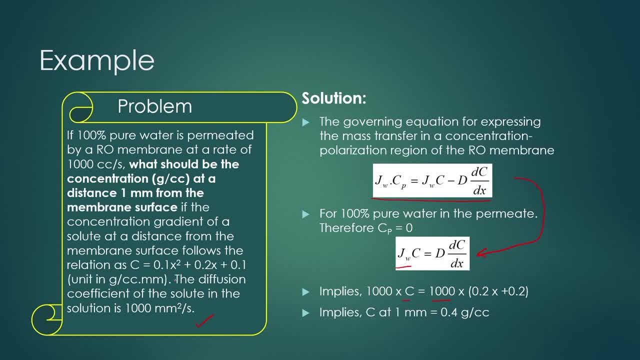 is given as per 0.1, what is that? after, you know, after derivative dc by dx, from this equation where concentration with respect to x is given here, so from this dc by dx that will be coming as 0.2x plus 0.2. 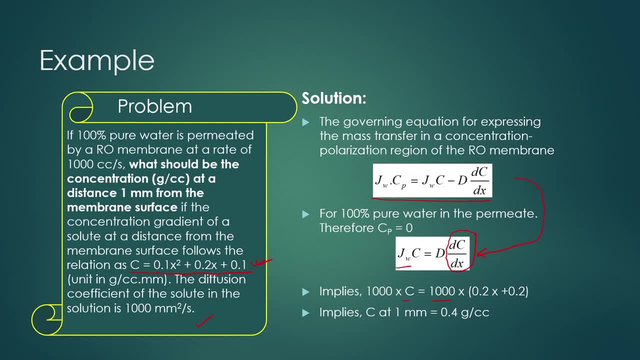 So at 1 millimetre that means x is equal to 1 millimetre, so C will be coming as 0.4 gram per cc from this equation. So I think you understood this problem here. how to solve. 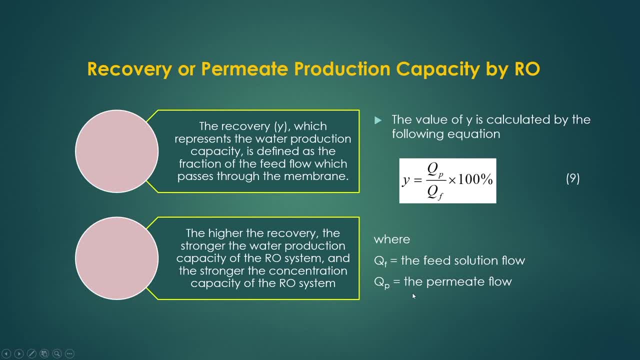 Then, coming to that, another important point here for this reverse osmosis system: how to actually calculate that recovery or permeate production capacity by that reverse osmosis system. In this case, if you are considering that recovery as y, which represents the water production, 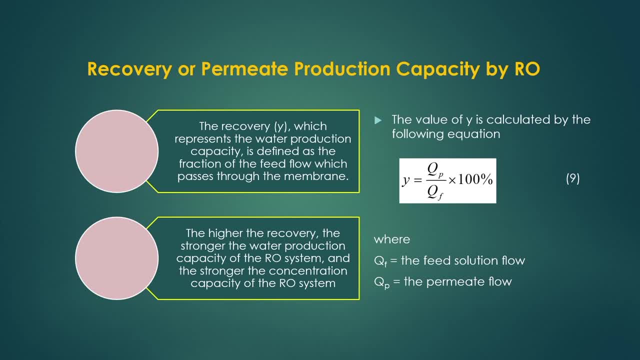 capacity, that means permeate solution capacity, which will be defined as the fraction of heat flow which passes through the membrane, And in this case 0.3 to 0.4 gram per cc. 0.2 to 0.5 gram per cc. 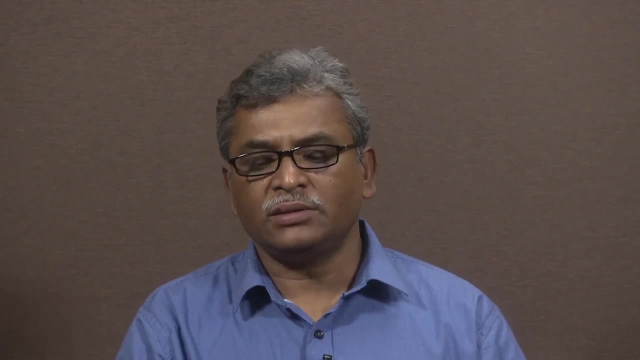 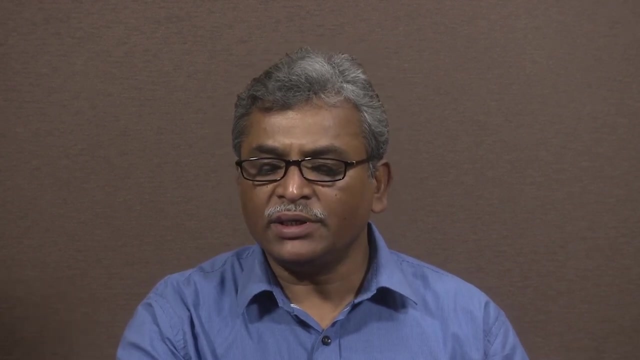 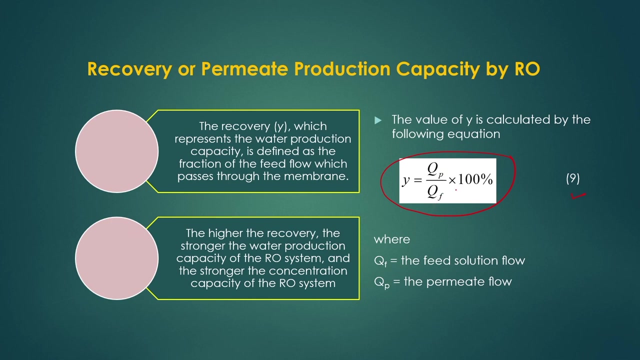 0.5 to 0.6 gram for each valve. Now if we know that permeate flow rate and the feed flow rate, then the value of recovery can be calculated by this equation 9.. So y will be: is equal to Qp by Qf into 100 in percentage. 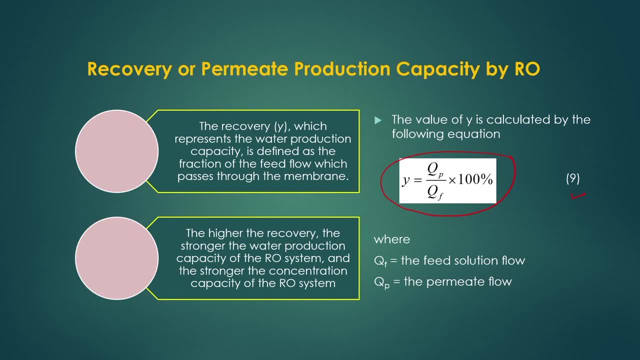 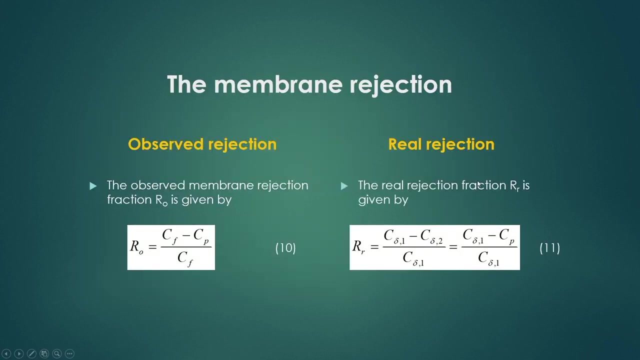 So this is called recovery percentage, and this recovery percentage will give you the capacity of this RO. Now, the higher the recovery, that means the stronger the water production capacity of the RO system and the stronger the concentration capacity of the RO system. So I think you understood this one and then another important factor that you have to. 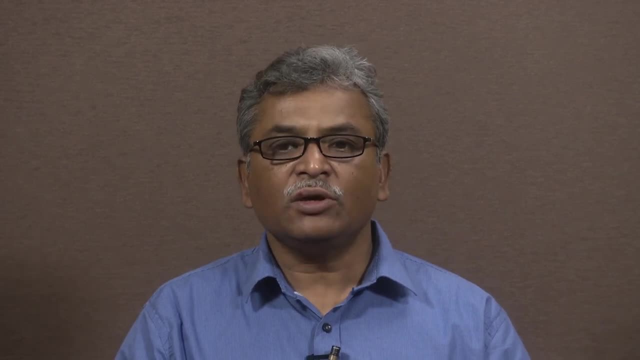 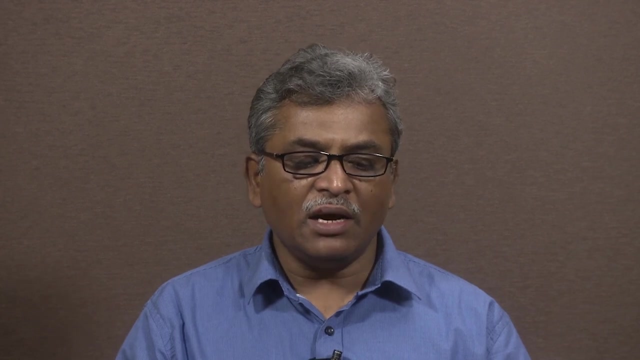 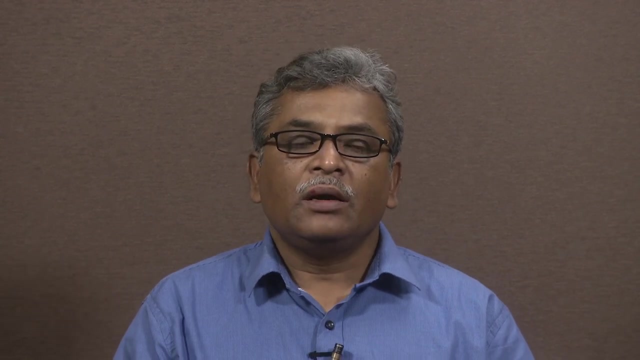 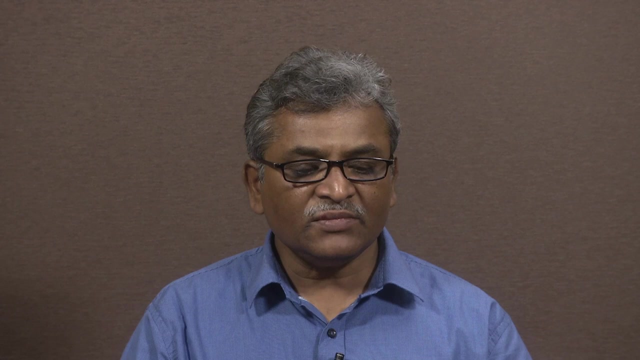 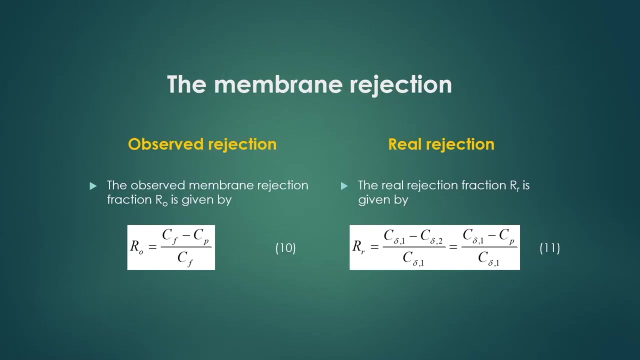 know it is called membrane rejection. By this also, this RO membrane separation process be assessed. In this case, Rejection is a one term by which you can interfere that reverse osmosis filtration process. There are two actually rejection: one will be observed, another will be real rejection. 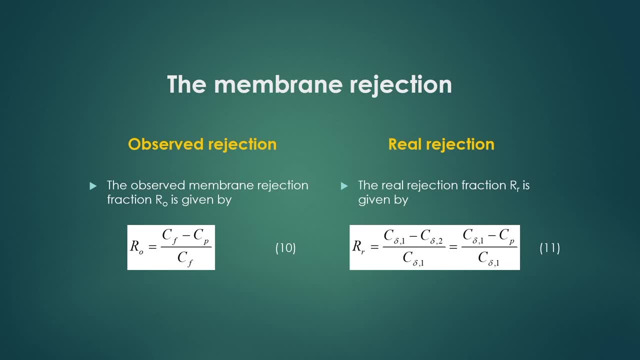 The observed rejection is basically based on that overall concentration in the feed and permeate side. So observed membrane rejection fraction can be expressed by this R? o. this is defined by this C f minus C p by C f. C f is the overall or average concentration in the feed solution. 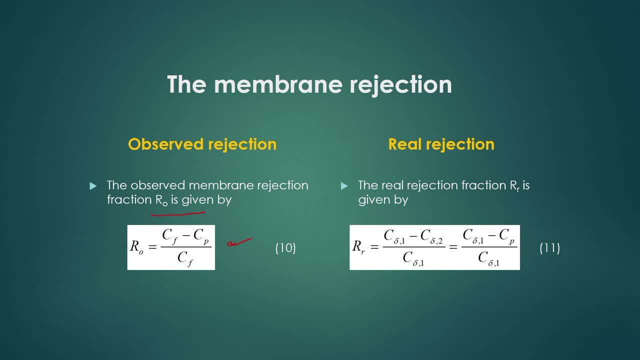 and C. p is the average concentration of the solute in the permeate solution divided by C- f. So this: what is the difference of that concentration in the feed and permeate? Permeate divided by the concentration of the feed, that will be called as that observed. 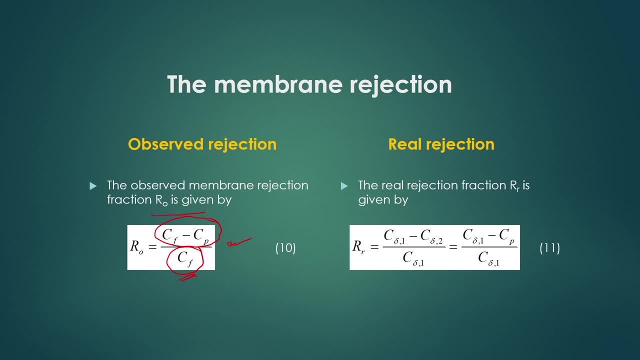 rejection, Whereas real rejection actually will be based on the what will be the concentration of that solute in the very nearer region of that membrane surface in the retentate side, And also what will be the solute concentration at the nearer side of that permeate solution. 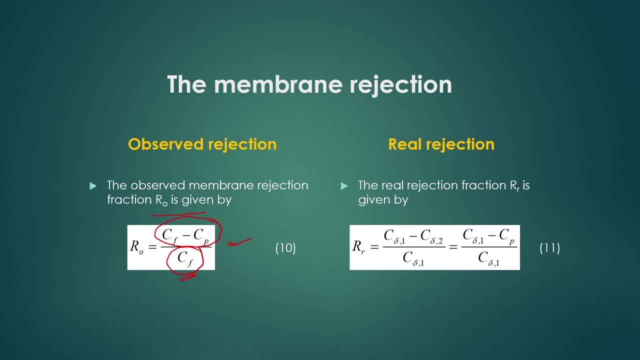 The permeate side of that membrane. So based on those concentration it will be considered as a real rejection. So real rejection fraction can be defined by R- r, So it will be C delta 1 minus C delta 2 divided by C delta 1.. 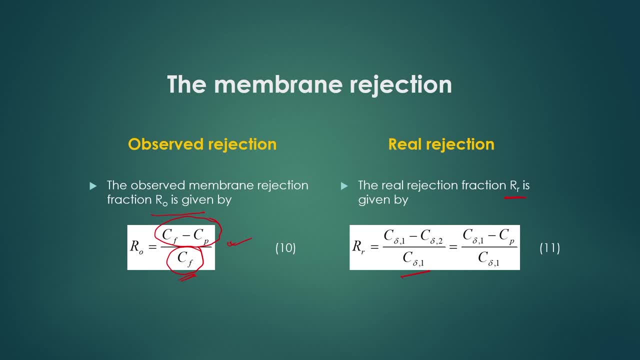 Here C delta 1, you know that at this concentration polarization region, very adjacent to the membrane surface, In the retentate side, what will be the solid concentration? and C delta 2 is the concentration of the solute at the permeate side, which is very near to the, you know, membrane surface. 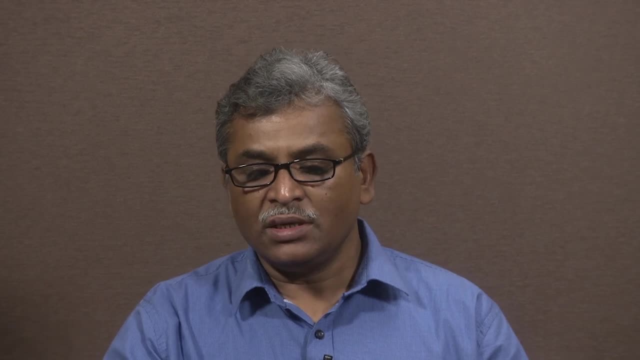 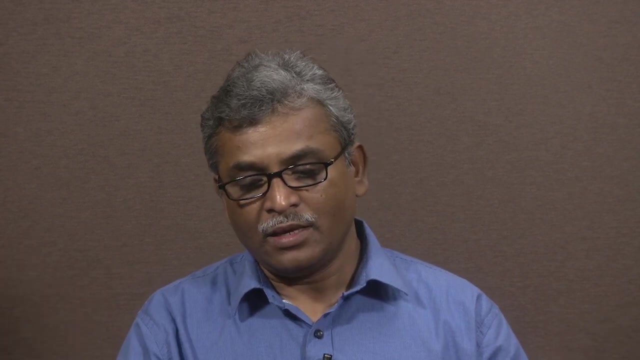 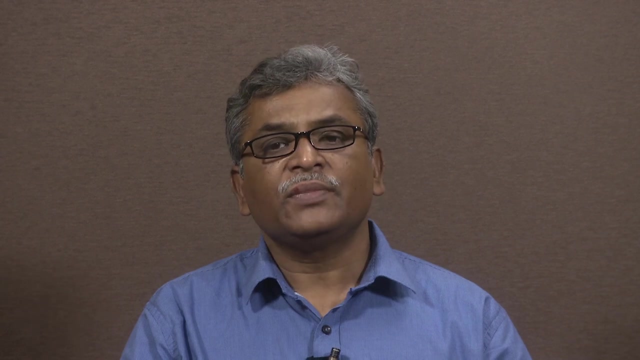 at that permeate side. So based on these you will be able to calculate what will be the real rejection Once you know that concentration at that side. So very difficult to actually calculate that concentration of the solute At that you know, you know surface of that, you know membrane, or at the concentration. 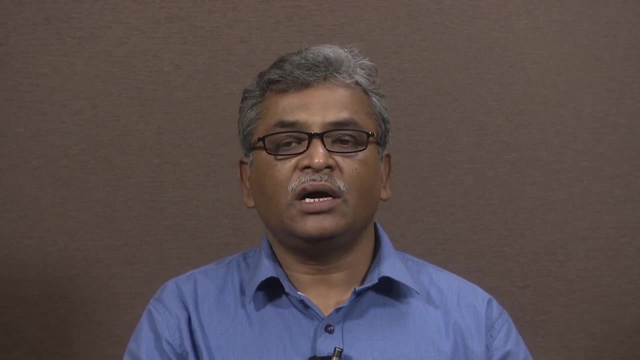 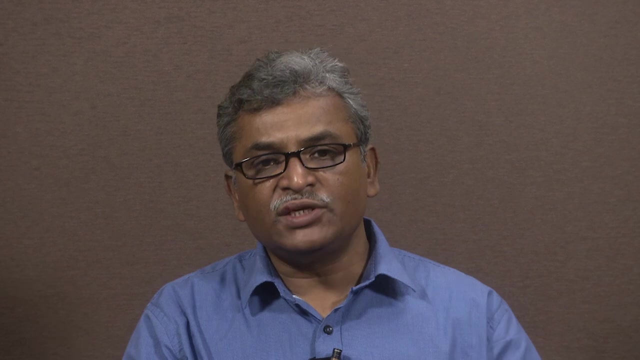 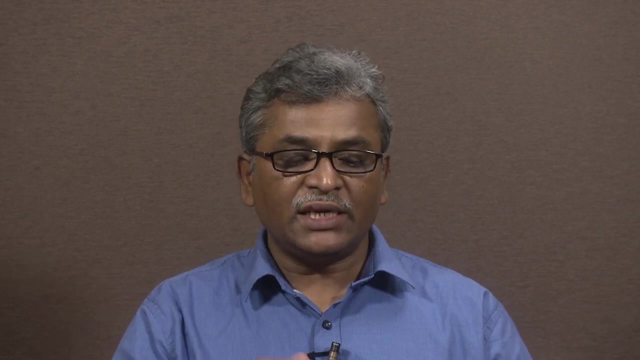 polarization region. So for that average concentration is taking by you know calculating its, that you know in the feed solution and also in the bulk solution at that permeate side what will be the concentration it is taking as a average. So in that case observed rejection is to be followed, for you know interpretation. 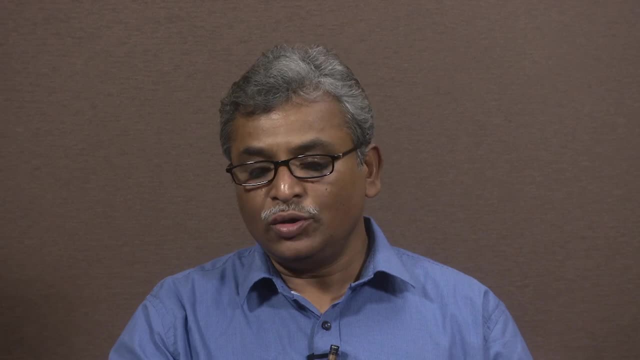 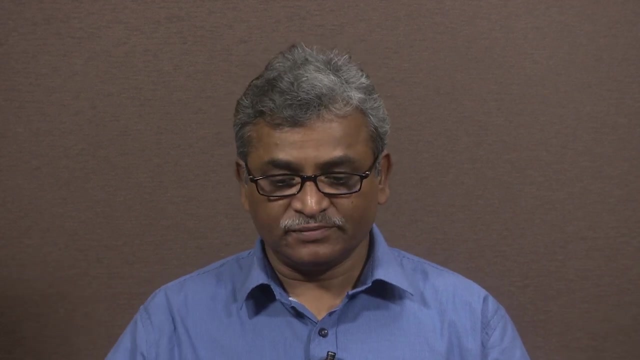 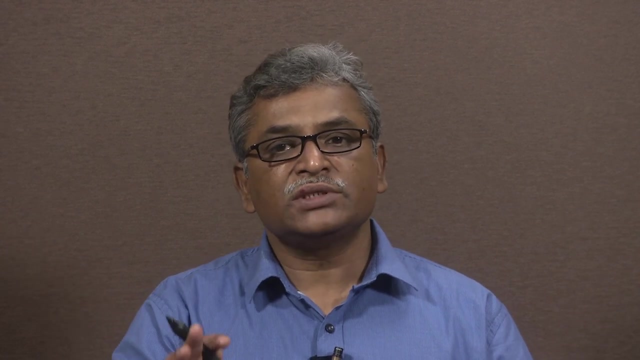 of that membrane That will be overall, whereas real, to be calculated. based on that, if you know that concentration at the surface of that membrane- Nowadays very sophisticated instruments are used to you know calculate that you know solute concentration at that nearer to that, you know membrane surface and based on which. 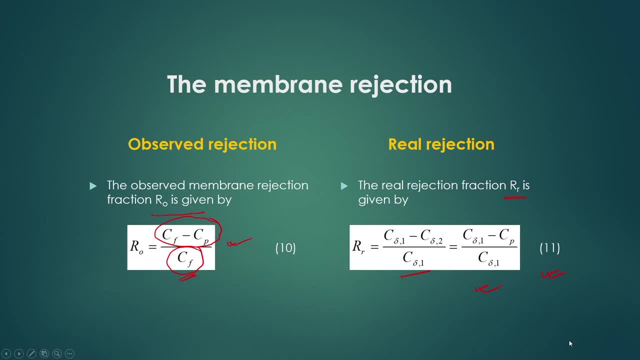 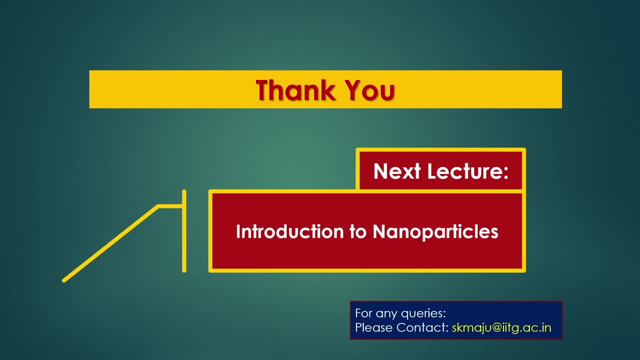 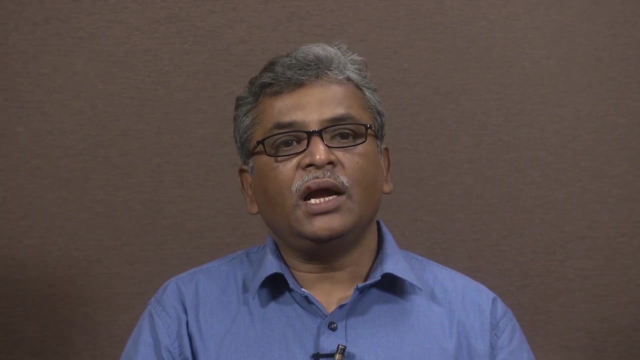 you will be able to assess that, you know, membrane efficiency based on this rejection of real condition. So I think you understood that. reverse osmosis system. Thank you. What is the difference between osmosis and reverse osmosis? What is the driving force? basically the pressure. 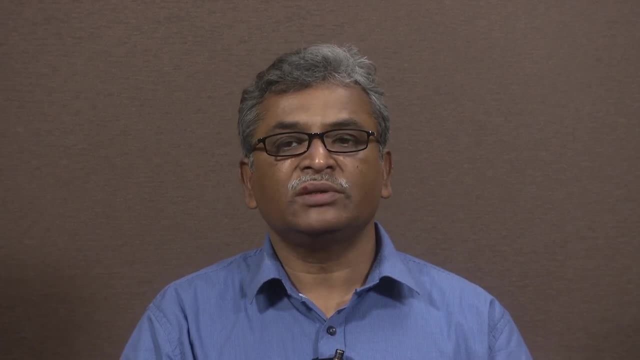 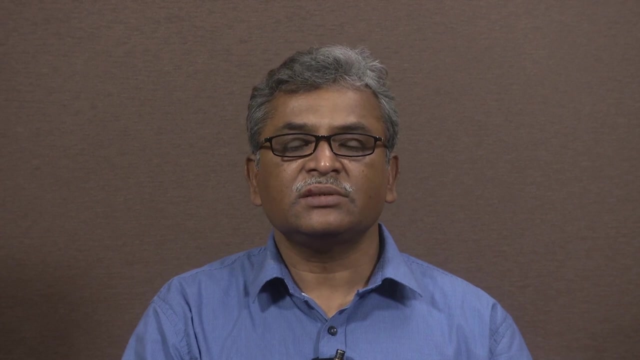 And also you have to assess that you know reverse osmosis. based on that, you know concentration differences And based on that concentration differences, you can assess that you know reverse osmosis based on that one-dimensional mass transfer model. 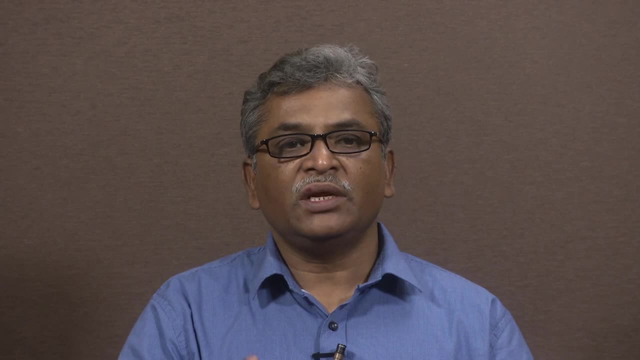 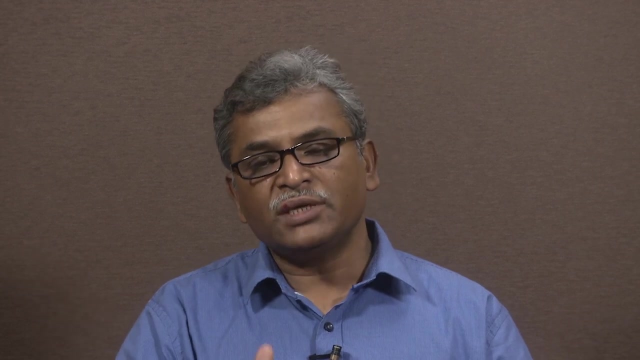 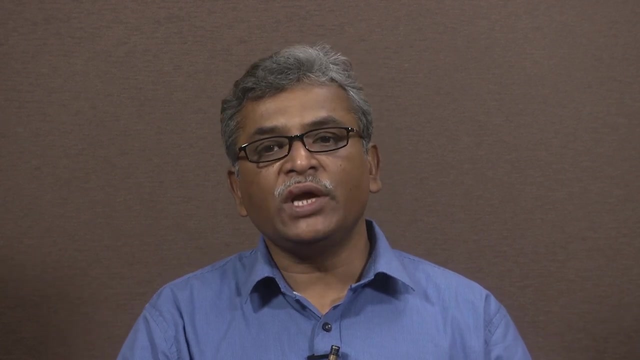 And for that mass transfer model, you are considering what will be the diffusion, what will be the net flux, And, based on that, what is the mass balance? and based on that mass balance you will be able to calculate what will be the you know concentration at a particular you know location. 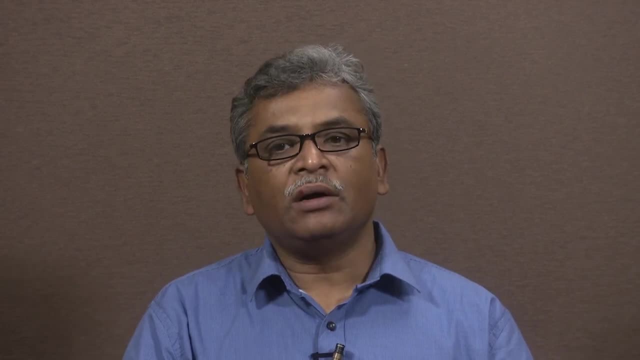 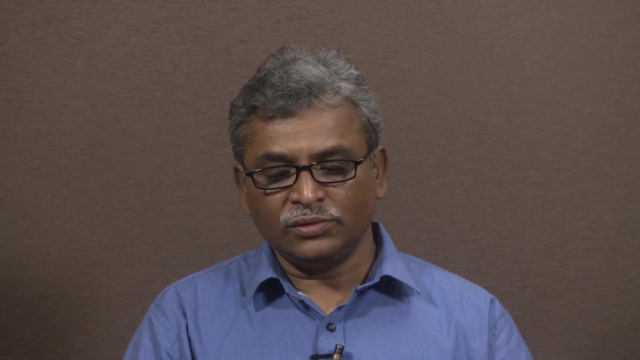 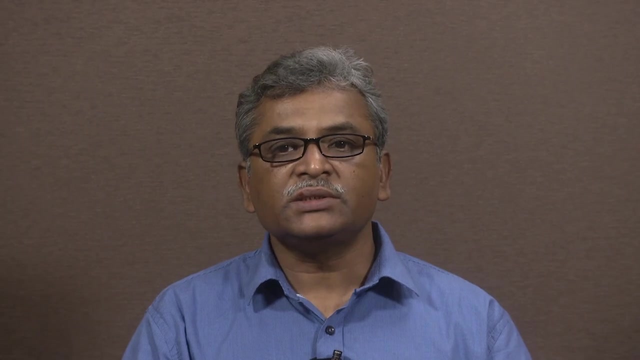 from that you know membrane. So I think you understood this. you know lecture here. what is the basic concept of RO membrane? In the next lecture onward we will try to discuss the different module which will be started And discussion of that. nanoparticles. 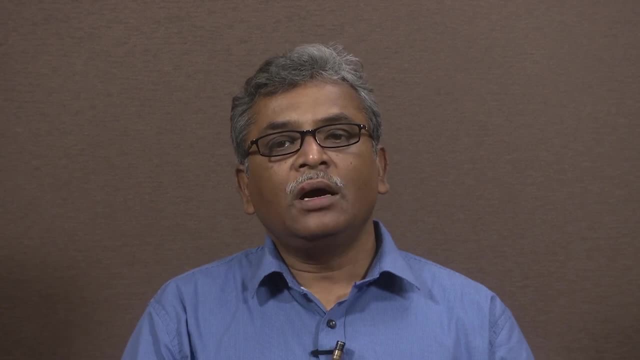 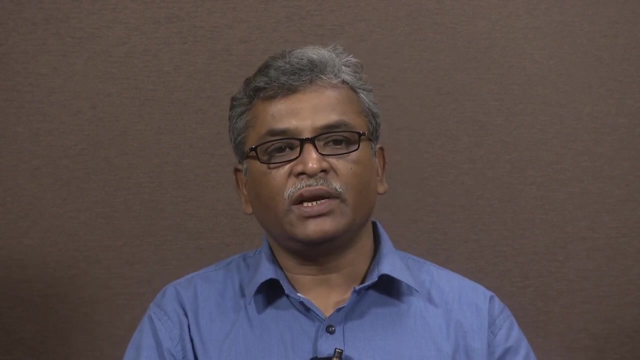 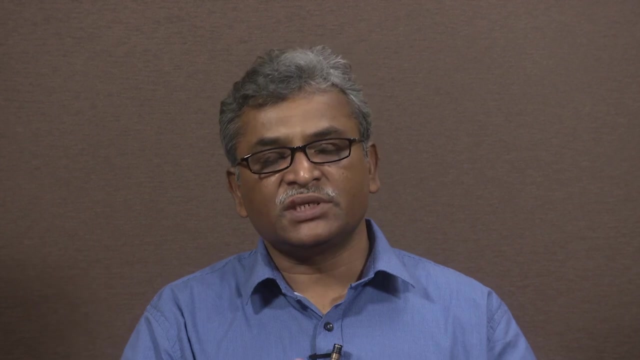 So till now we were discussing about. you know that you know microparticles and also that coarser particles, conventional particle size and how to separate from that slurry by different techniques. Also that some you know hydrodynamics, frictional pressure drop, even some material characteristics. 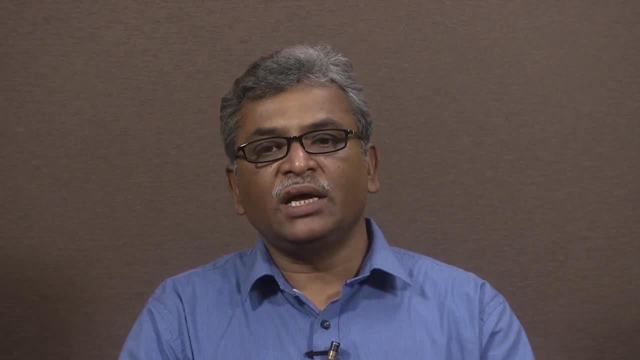 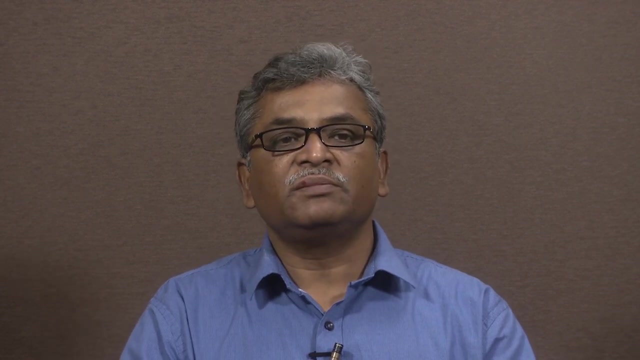 all those things. Now, next module onward, it will be there. you know some, you know. introduction to that: nanoparticles, nanosized particles. What is the basic concept of that? nanoparticles? where that nanoparticles are, you know, used? 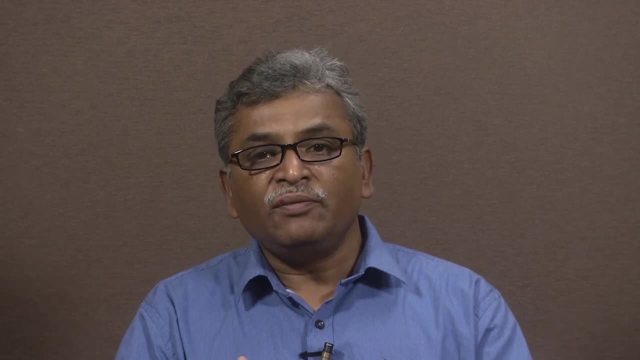 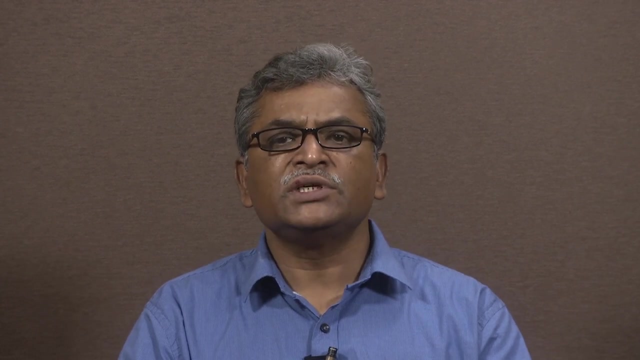 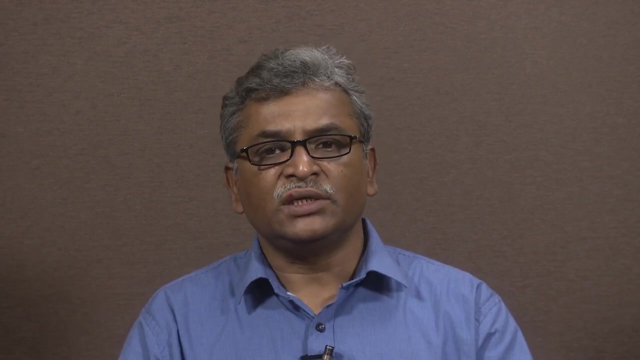 why those nanoparticles are so important nowadays. What are the different characteristics of that nanoparticles based on which that nowadays industry look into the process? intensification, based on this nanoparticle systems for various application to get that you know. enhancement of that yield of the reaction, even some other.